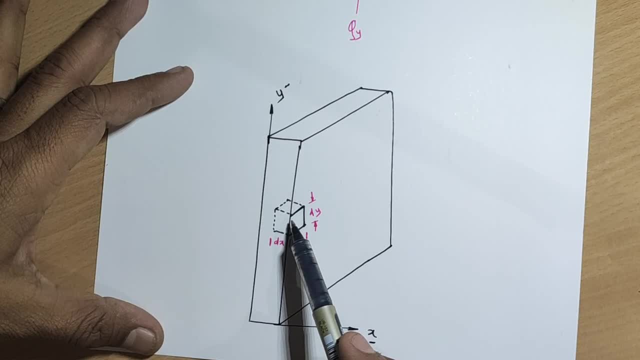 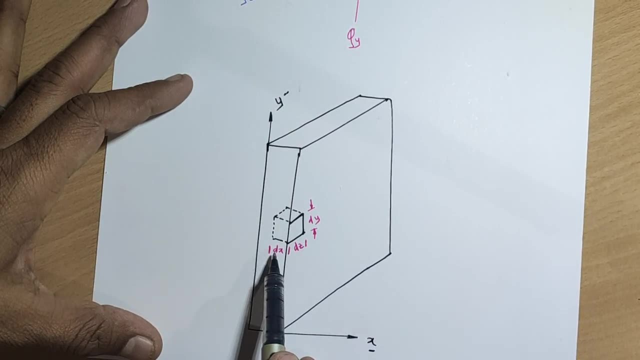 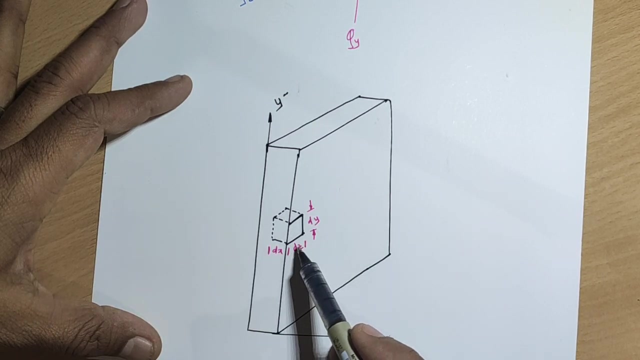 element. This is a small element on which I am going to derive an equation, and then from that I am going to derive the equation for complete wall. For this small element, the width in x direction is dx, in y direction the width is dy and in z direction the dimension is dc. 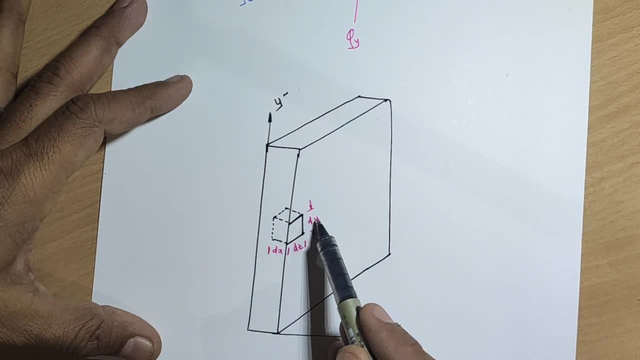 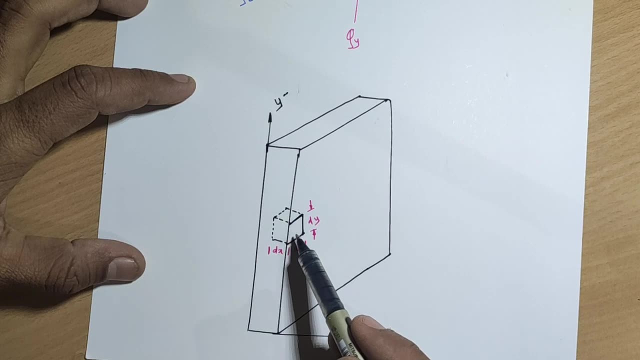 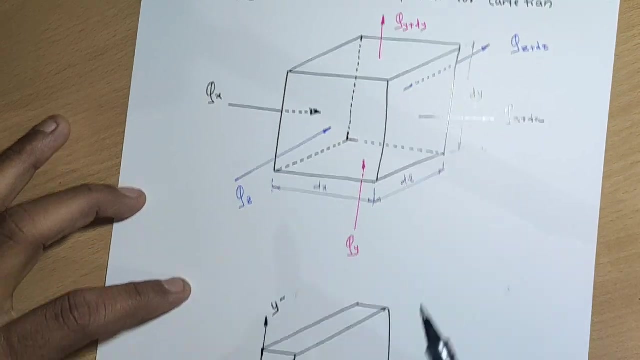 So for this particular small element, dimension is dx, dy, dz. These are the three sides of this element and for this I am going to derive an equation. Now, this element, if you get expand and draw the figure, I will see this particular figure. So this figure is nothing but this. 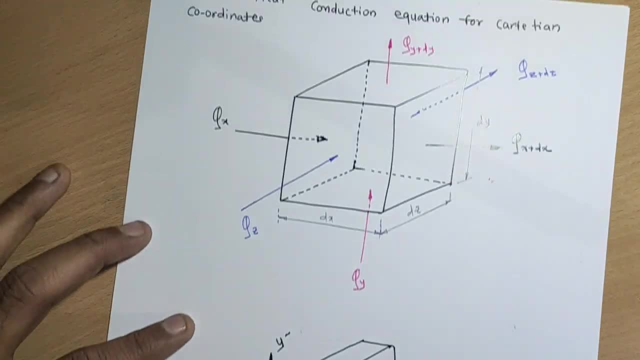 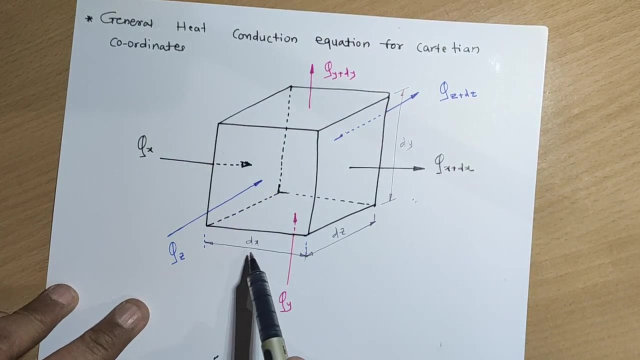 element which has a dimension dx, dy and dz. For this figure. let us see the dimension shown here. this is the cube which we have considered, In that x direction, dimension is dx, in y direction, dimension is dy. in z direction, dimension is dz. So this is the element which we have taken from wall which has a dimension dx, dy and 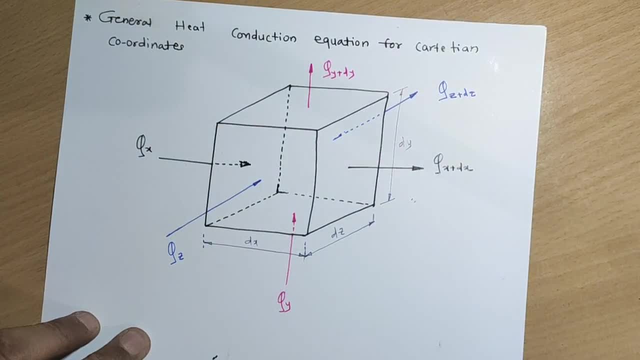 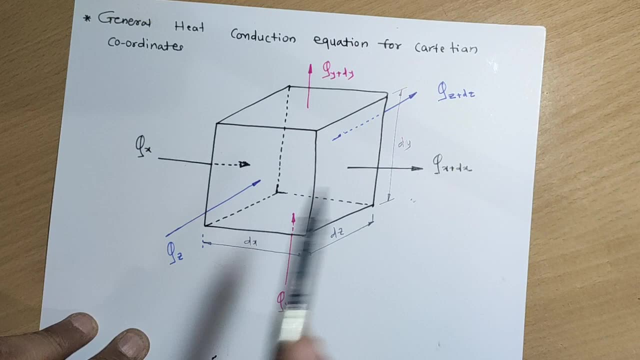 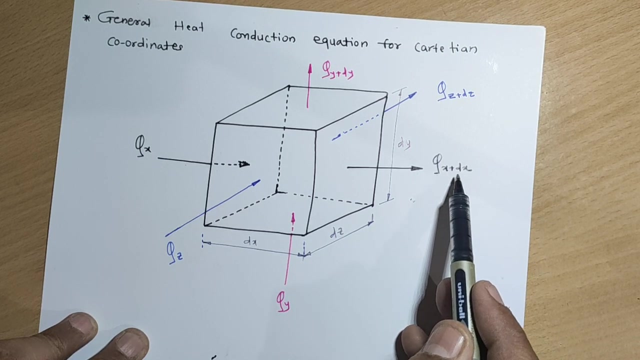 dz. For this particular element. the heat interaction is there from three sides. Heat entering in x direction is qx. So this is x direction, horizontal direction. Heat entering in x direction is qx, Heat exit from x direction is qx plus dx. So x plus dx is suffix here and here suffix is x. So entering it is qx, exit it is qx plus. 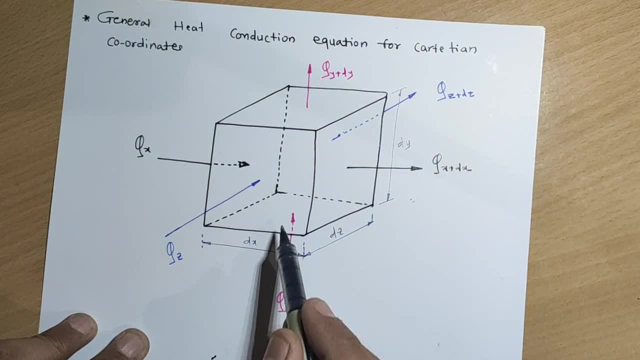 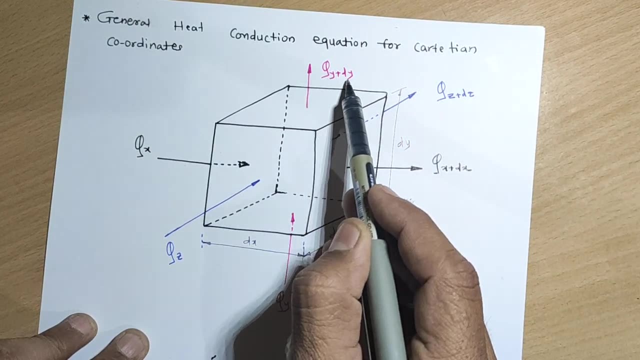 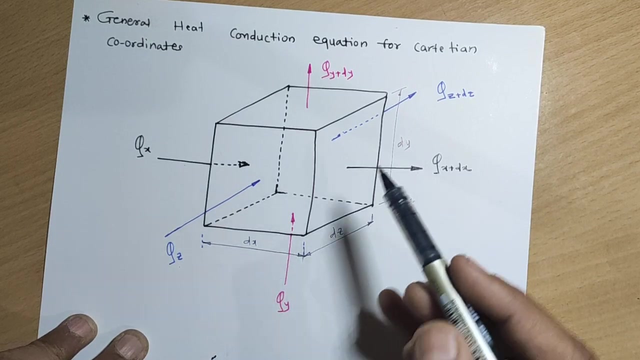 dx Heat entering in y direction, which I have shown by red color. Heat entering in y direction is qy, whereas heat exit in y direction is qy plus dy. Similarly, in z direction heat entering is qz. This is the heat entering in z direction qz and heat leaving in z direction. 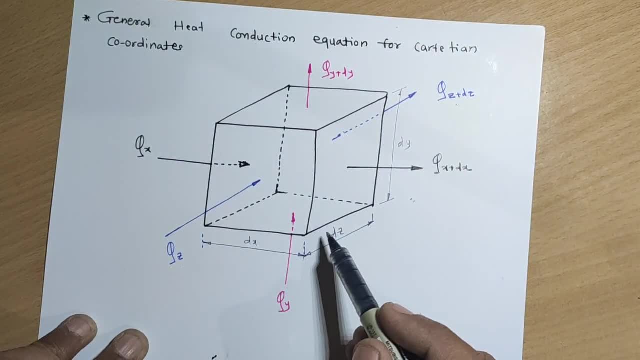 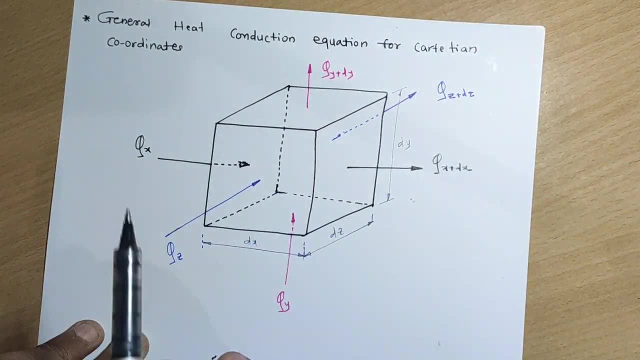 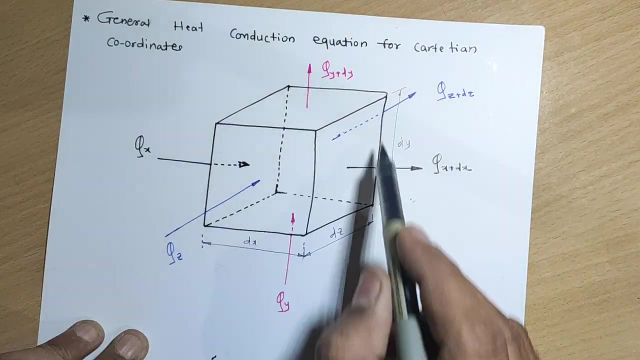 is qz plus dz. So these are heat interaction which is happening with this particular element in three direction. So in x direction, y direction and z direction heat is entering At the same time in x direction, in y direction and z direction heat is leaving. So I have to derive general heat conduction. 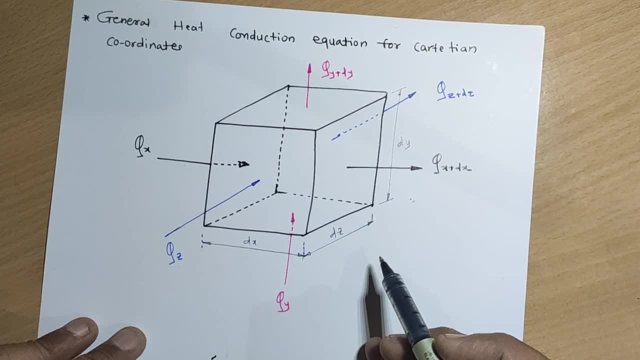 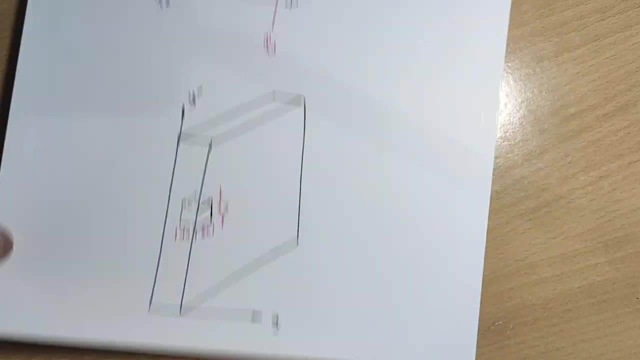 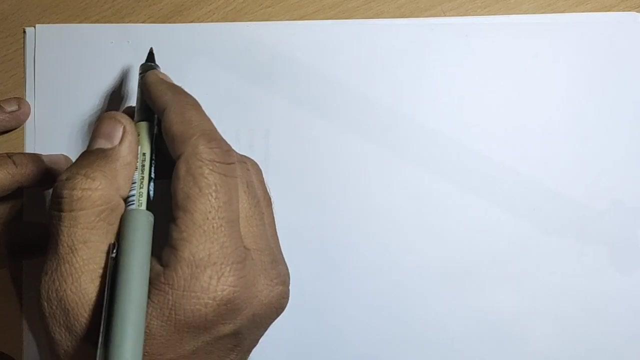 equation for this element. For this, first of all, I am going to consider the energy balance equation. So let's write an energy balance equation first of all. So the Energy balance equation for this I can write like this one. So this I am writing according to: 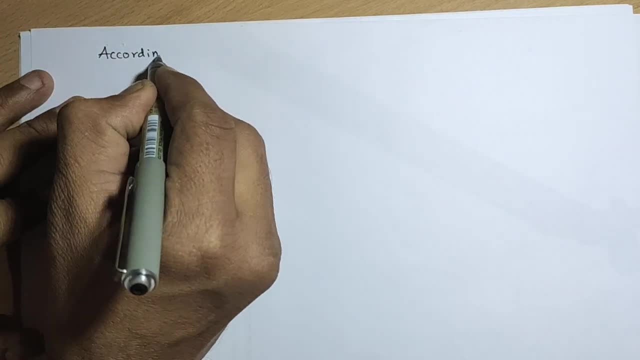 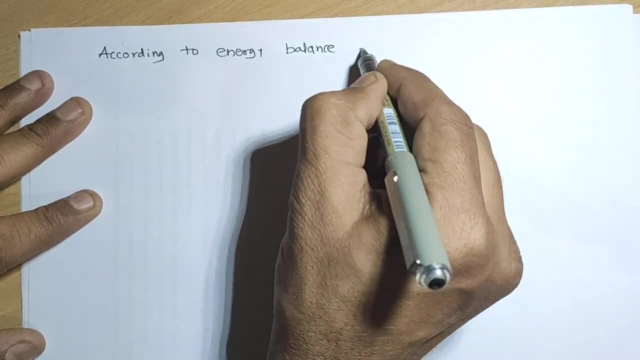 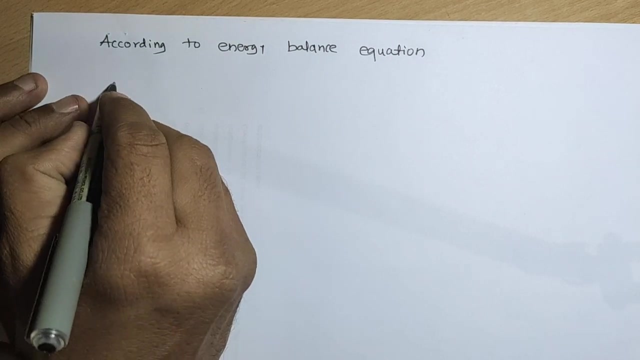 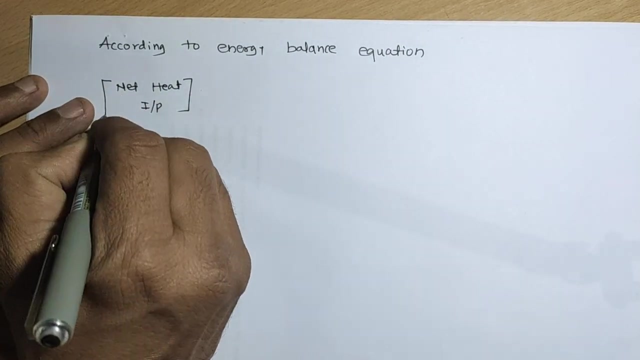 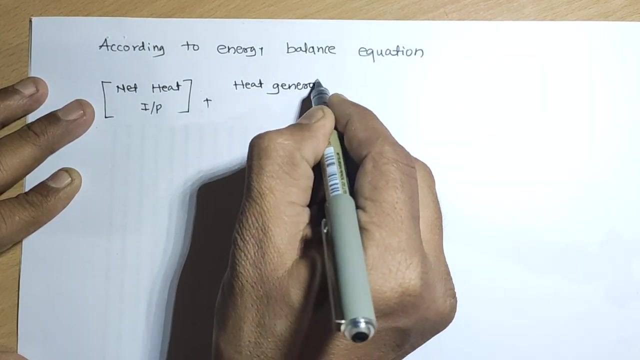 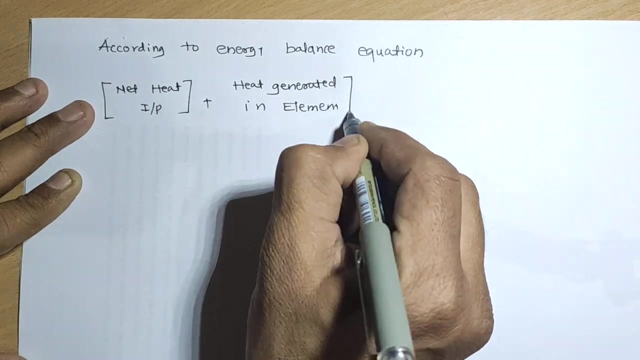 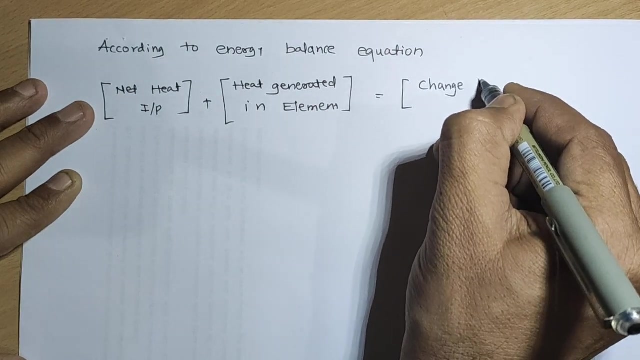 energy balance equation. According to energy balance equation. According to energy balance equation, Net heat input einen net heat input input, net plus heat generated in the element. heat generated in element. this is second. so summation of these two is nothing but change in internal energy, changing internal energy. so what we? 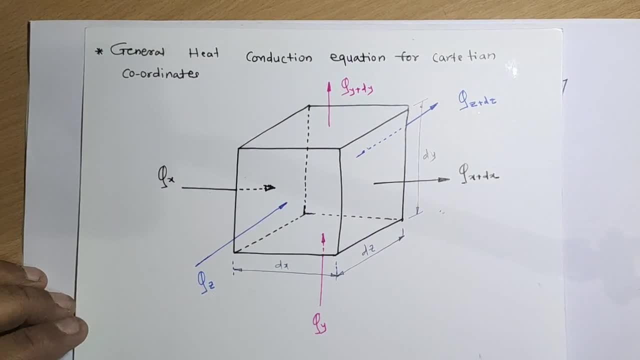 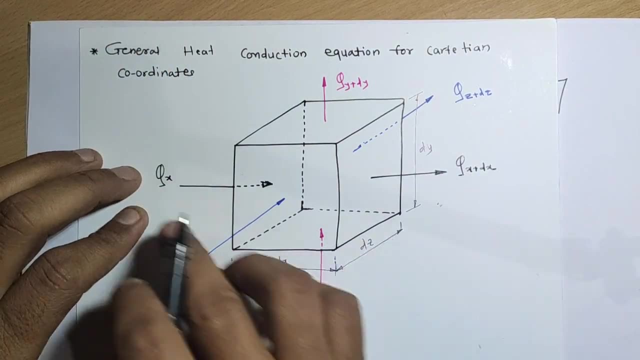 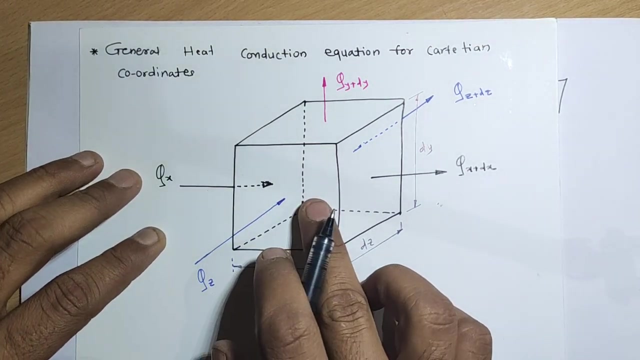 have written this equation. we have written for this particular element. so for this element, if i consider energy balance equation, net heat input is the heat input in all three direction plus heat generated in the system. if i make summation of net heat input and heat generated in system, that will give you change in internal energy of the system. that's. 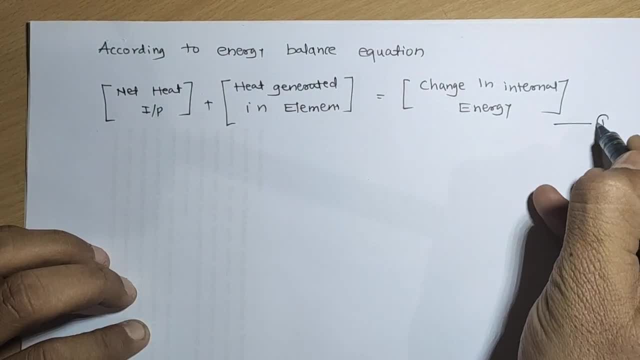 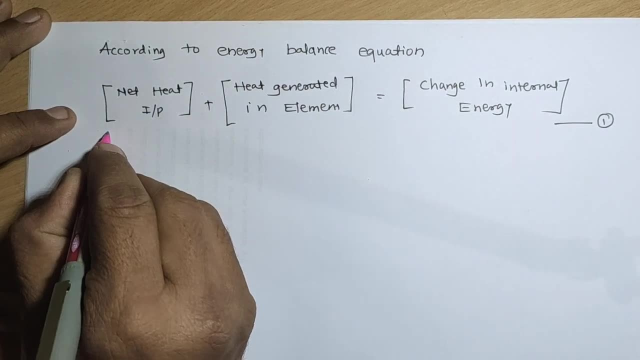 what energy balance equation we have written. let's consider: this is the equation number one. now what i am going to consider this equation, i am going to divide it into three part. what are the three part? the first part is this one, so this is part number one. part number one is net heat input into the 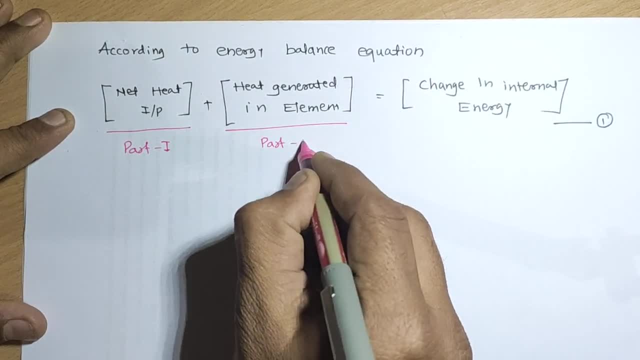 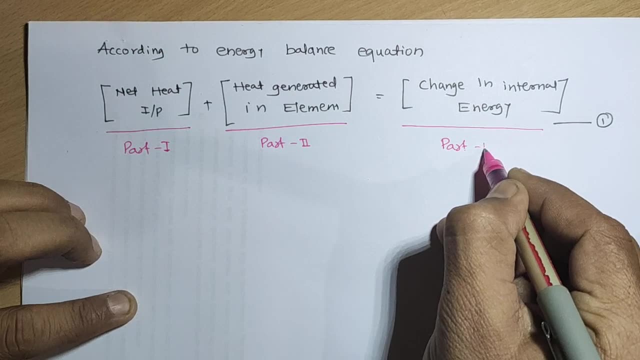 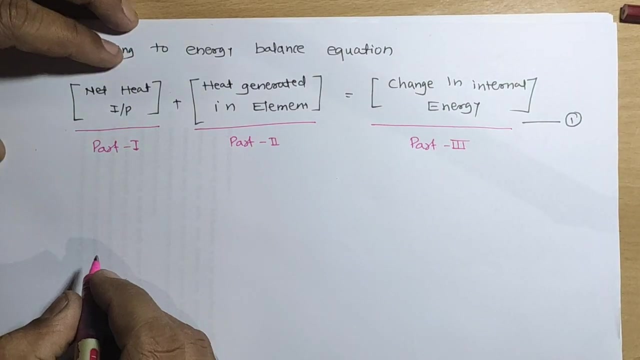 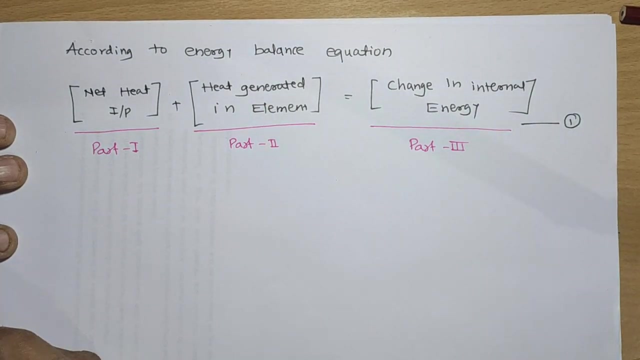 element. part number two is this one which is heat generated in elemennt, and next is this one part three. so this equation number one, i have divided into three element, as part number one, two, and now what i am going to do is i am going an equation for all these three parts and i am going to put one by one into equation number one. 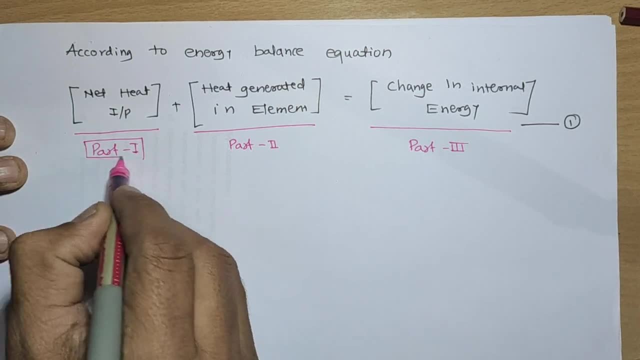 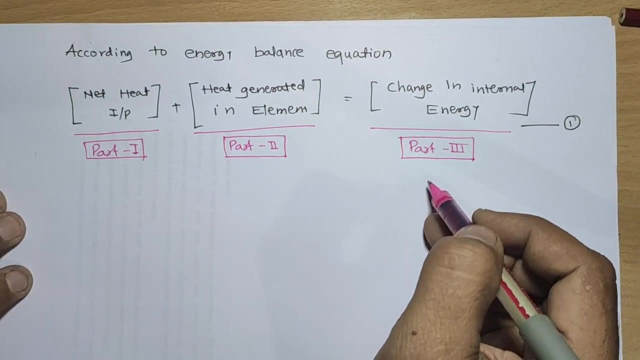 so means, first of all i am going to derive equation for part number one, then i am going to derive equation for part number two and finally i am going to derive equation number, my equation for part number three. and all these three equation i am going to put into equation number one to get. 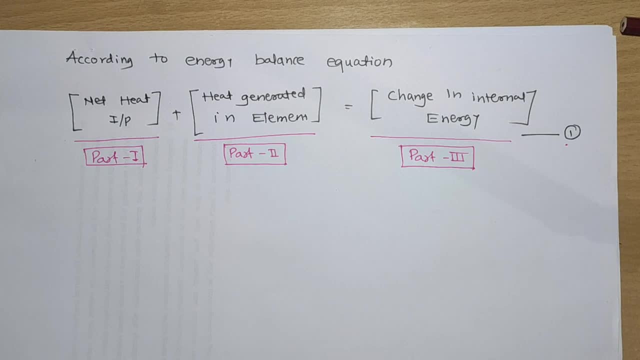 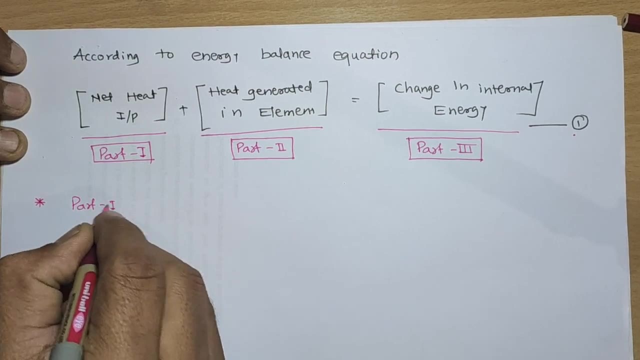 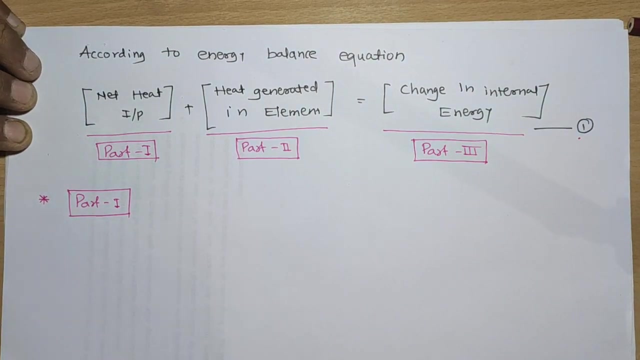 the final equation. now let's derive one by one. let's consider a part number one first of all. so i am going to consider a part number one first. and we chose that: the net heat input. now what i am going to write is net heat input in all three directions. let's consider net heat input in all. 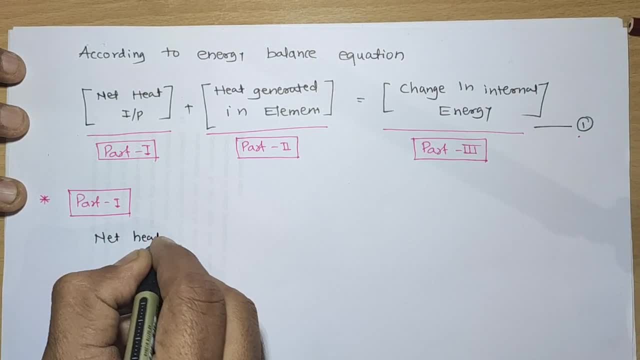 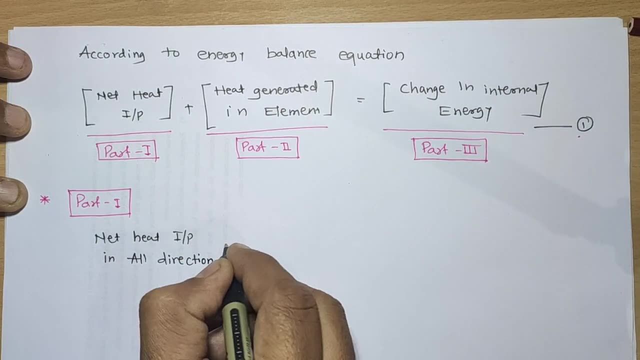 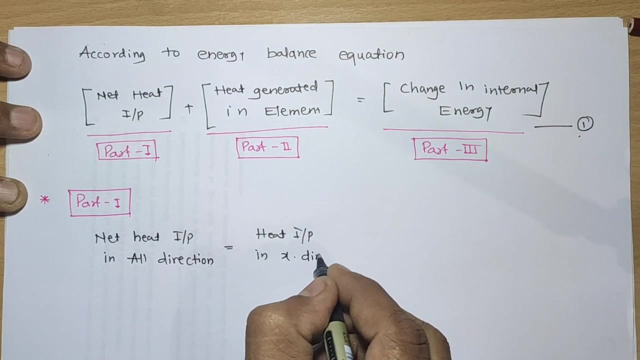 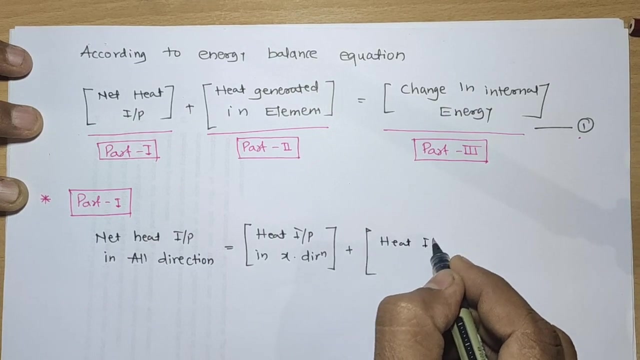 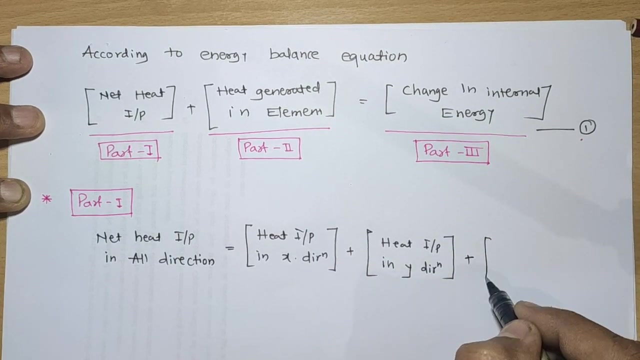 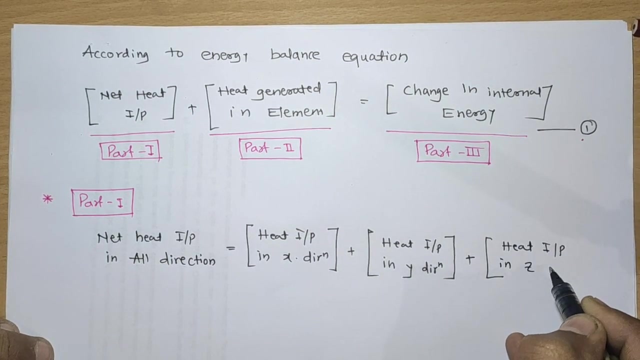 three direction. so net heat input in all direction is nothing. but i can write heat input in x direction, so i have three direction. so this is heat input in x direction, next is heat input in y direction and third is the heat input in z direction, so heat input in z direction. so i consider three direction and the net heat input in. 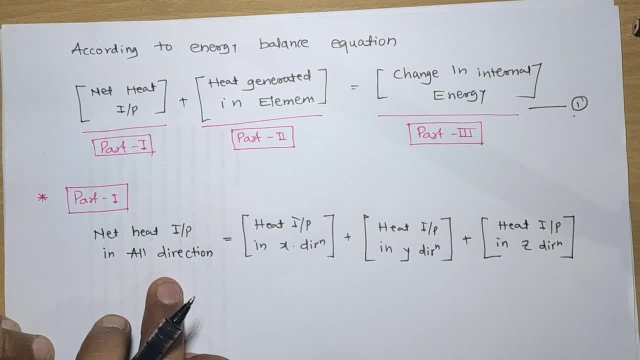 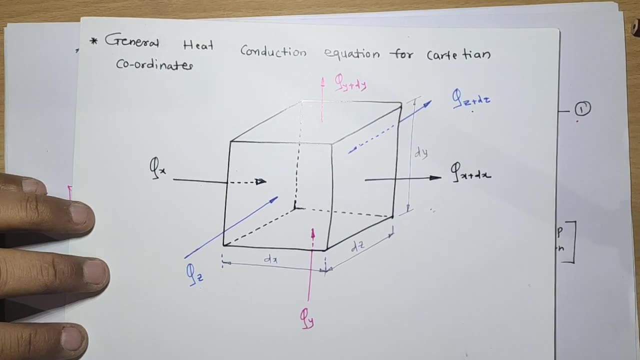 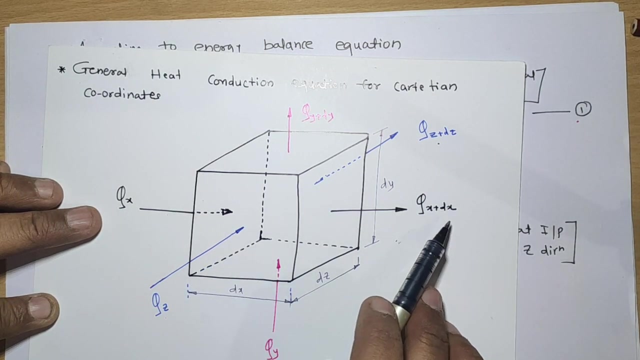 x, y, z is nothing but total heat interaction to this one. so this one i can write net heat input in x direction. let's refer this particular figure. in this figure, if i consider x direction, x direction, entry is qx, exit is qx plus dx. so if i take a difference between these two, input is qx output. 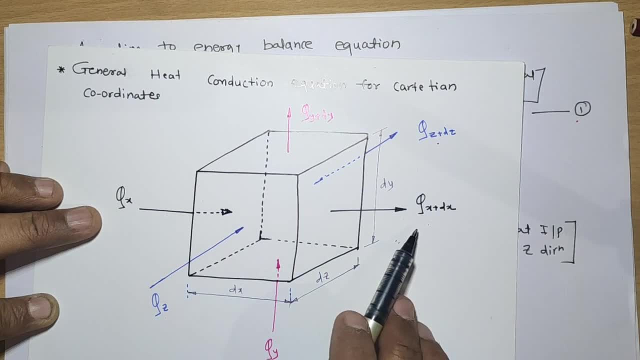 is qx plus dx. if i take a difference between these two, that will be net. heat input in x direction. in y direction, qy is entering, exit is qy plus dy. if i take difference between these two, that will become net. net means what the difference between 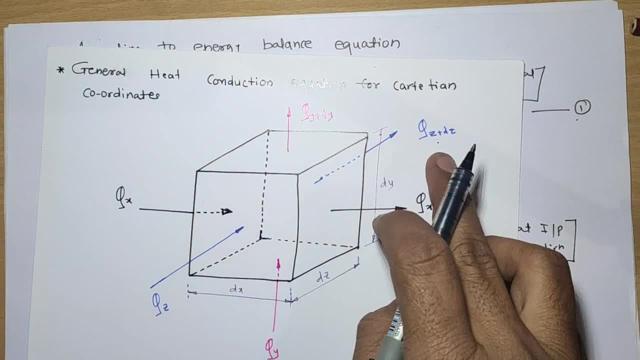 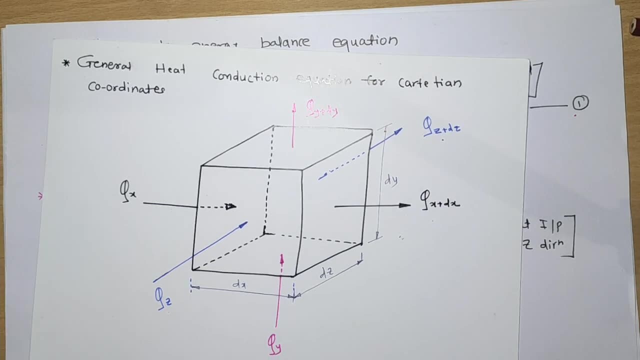 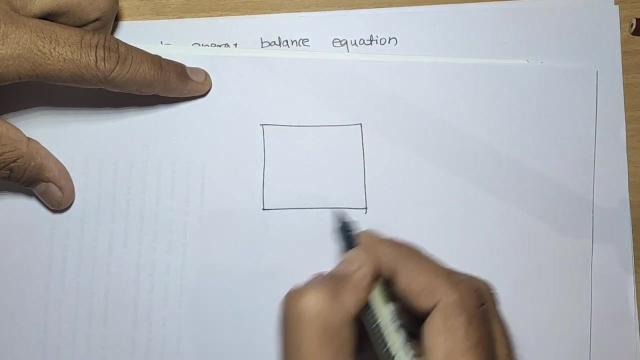 these two in z direction. qz is input and qz plus dz is output. so difference between these two will be the net heat input in z direction. okay, this has came from principle. i will show you simple example. if i take this as element in this element, if hundred joule amount of energy is coming in, 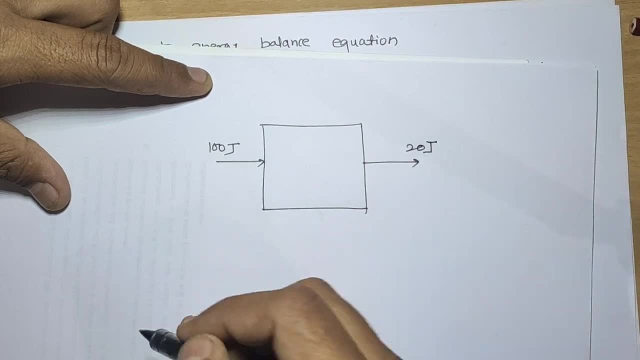 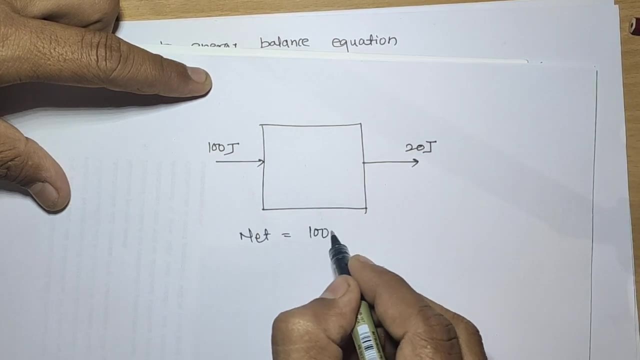 and exit is. let's consider an energy that goes in this direction, so let's call it. energy is generated in. let's consider 20 zone, so 100 is coming and exit is 20, so what will be net hit input? in this case, net hit input will be 100 minus 20, that is entry minus exit, and we'll get 80. so this is called as. 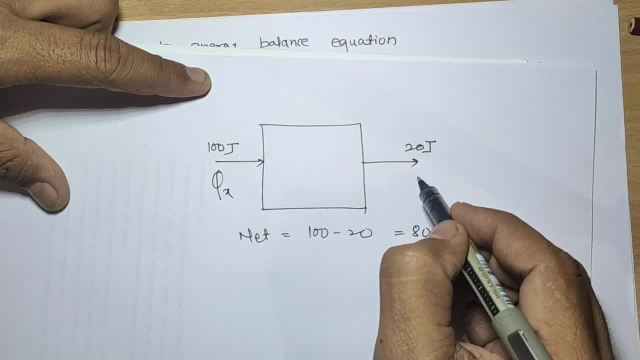 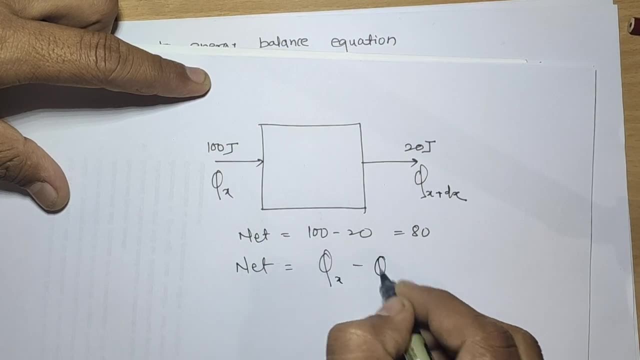 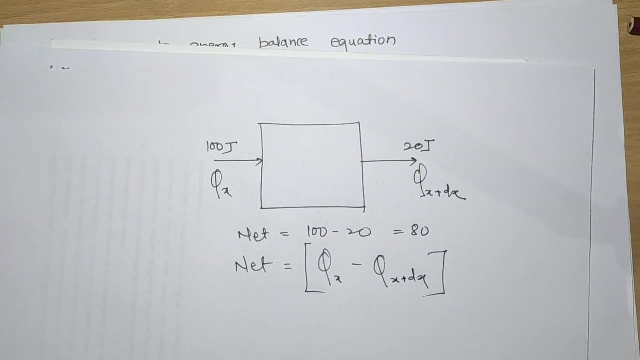 net: hit input. similarly, if qx is input and exit is qx plus dx, then what will be net? net will be qx minus qx plus dx. so this is net. hit input in x direction. similarly, i can write for y and i can write for z direction. okay, so by this principle, by this principle, let's write first. 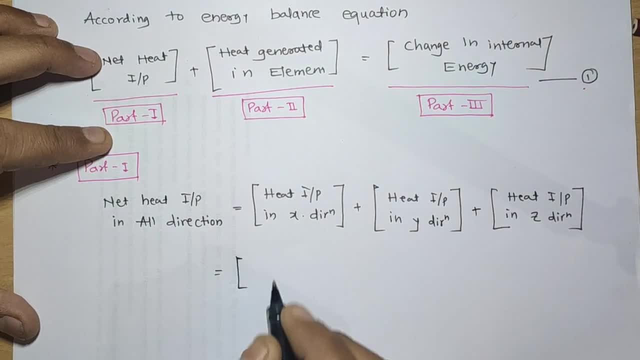 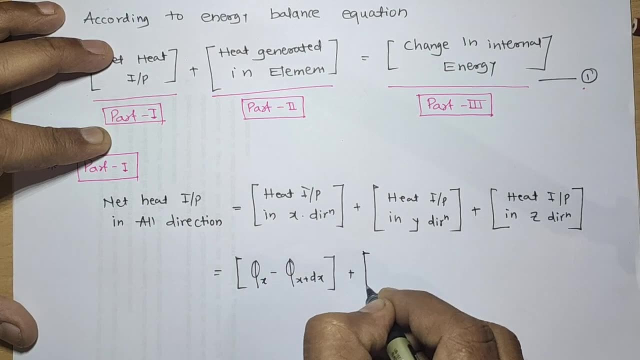 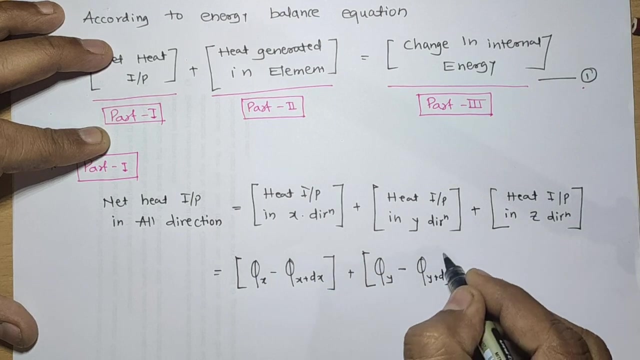 of all for x direction. so for x direction, as i told you, that is qx minus qx plus dx, that is net hit input in x direction plus net you didn't put in y direction. that is qy minus qy plus dy, plus in z direction. similarly, i can write qz minus qz plus dz. that is the equation. 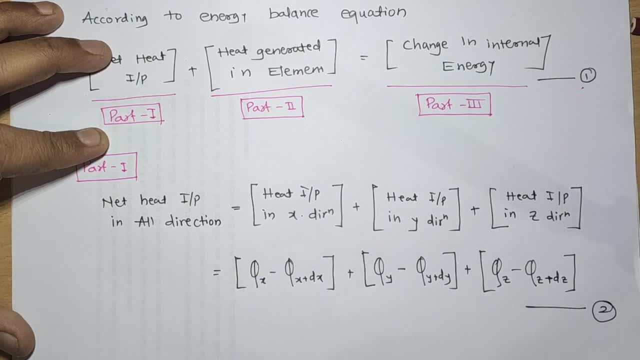 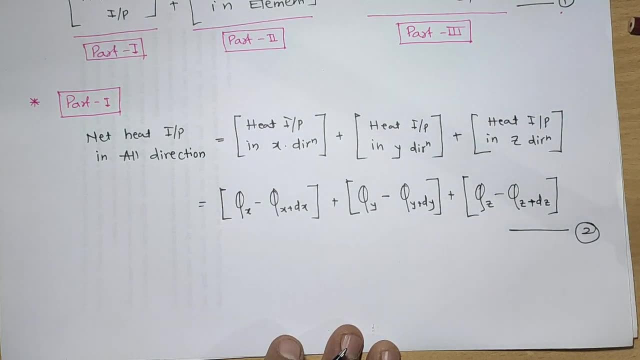 we have got, and let's consider, this is the equation number two. so we have got an equation number two. now next task, what we have to do is we have to find out an equation for equation for net hidden: put in x direction, net hidden y direction, net hidden: put in z direction, and then 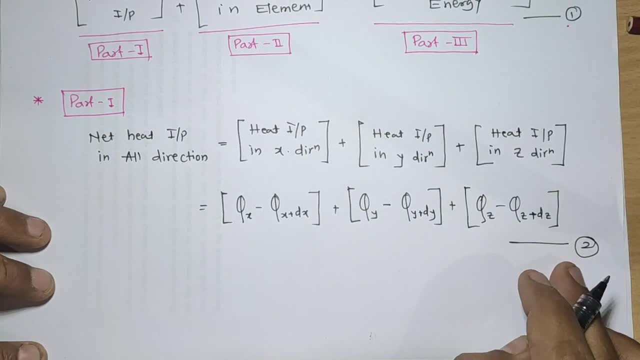 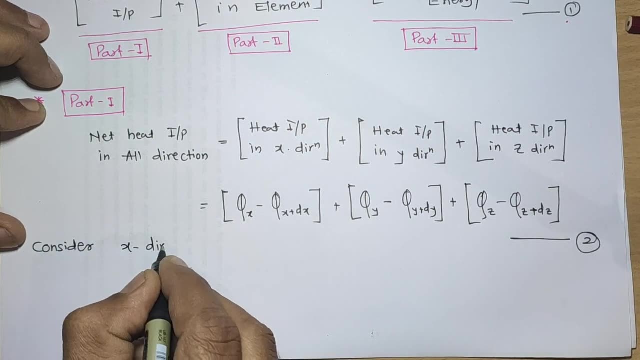 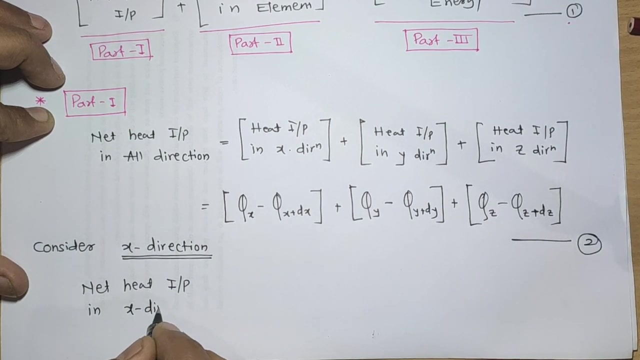 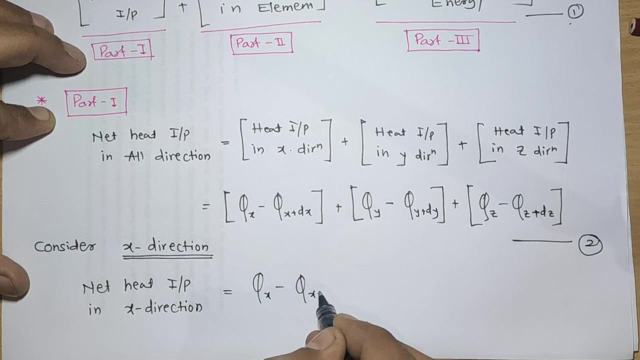 that equation we have to put in equation number two to get the final equation. so now consider, consider x direction. so first of all i am going to derive an equation for only x direction. so for x direction, for a x direction, net heat input in x direction. x direction, which we have, equation as qx minus qx. 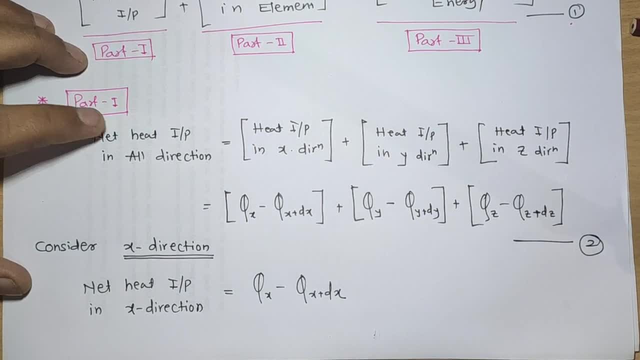 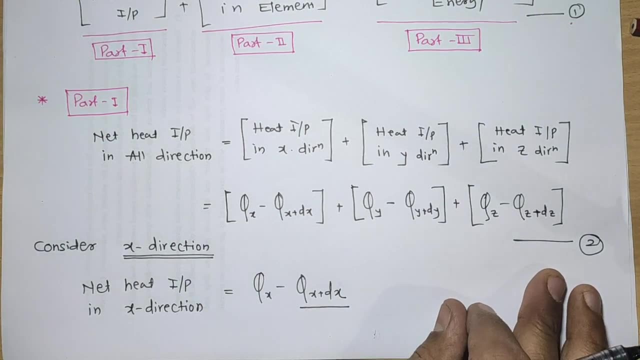 plus dx, that is the net heat input in x direction. now what i am going to do is i am going to expand this term according to taylor series. that is, from the mathematics, from the knowledge of mathematics, you will be knowing what is taylor series. so by the taylor series, i am going to expand this one. 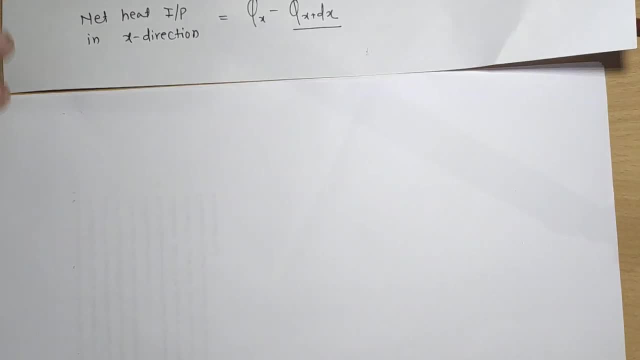 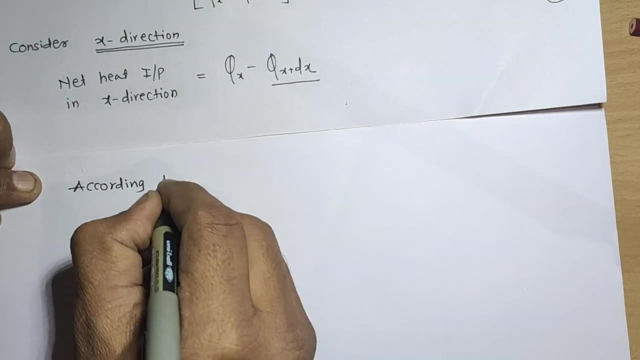 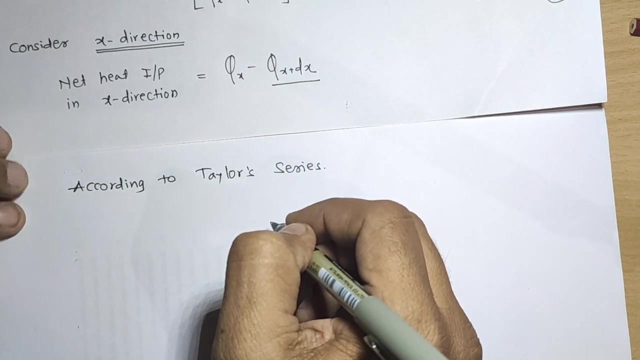 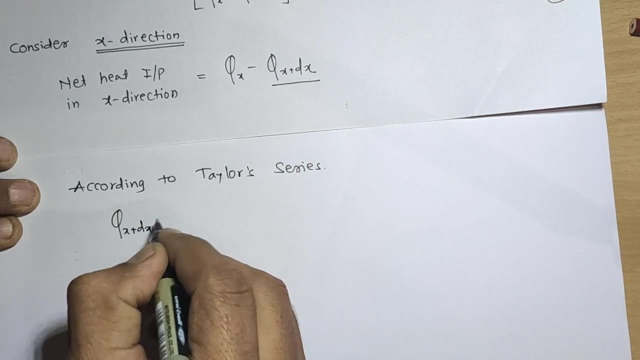 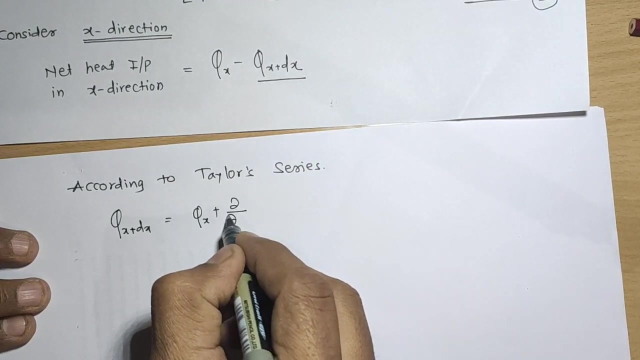 so let's expand this. so what i am going to do is according to taylor series. according to taylor series, this is from knowledge of mathematics that you might be studying in m3. okay, so qx plus dx. that can be expanded by the stellar series as qx plus d of dx, qx. 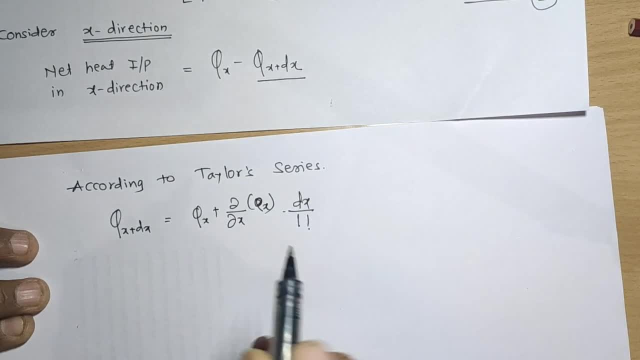 dx 1 factorial. so what we have done is this. i am going to expand. if i am knowing qx, i can find out qx, 1 factorial, x plus dx by using taylor series which says that qx plus dx is nothing but qx plus d of dx, qx into dx upon 1 factorial plus the next term. this is the first term we have written. 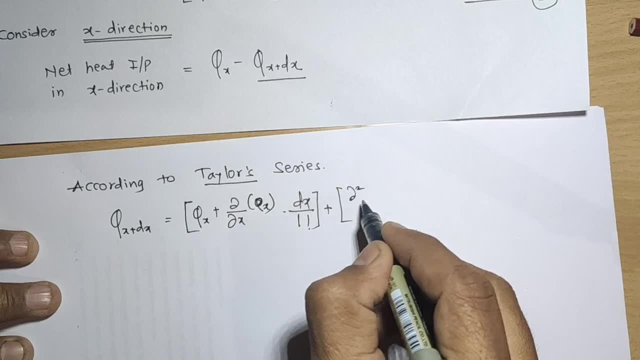 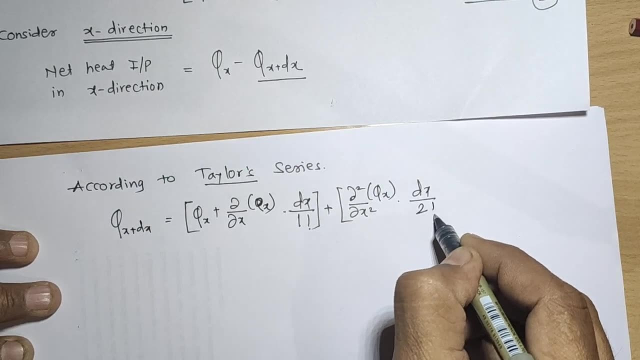 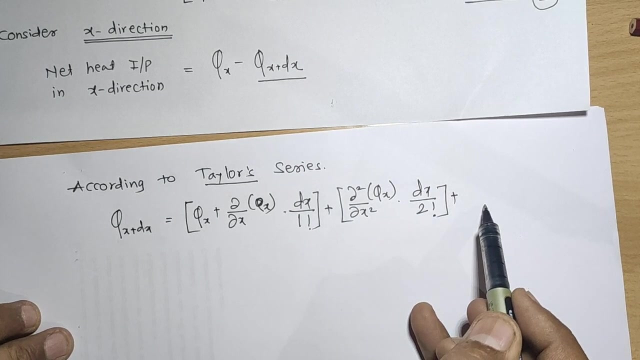 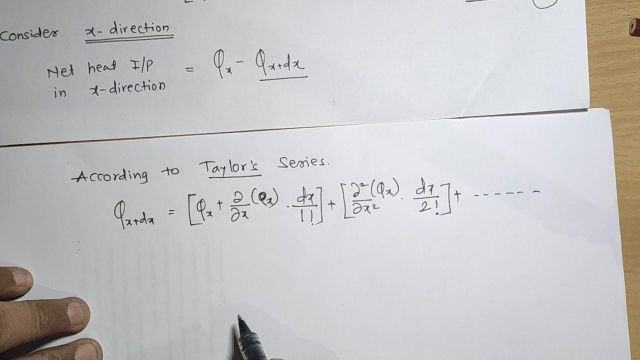 next term is the d square upon dx, square of a qx into dx upon 2 factorial. the third term i can write as d cube by dx, cube, qx, dx, 3 factorial. next there will be 4 factorial, 5 factorial, like that. we can go on expanding, okay. so this we are. 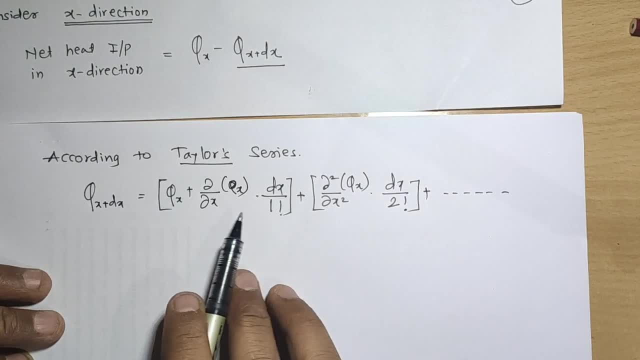 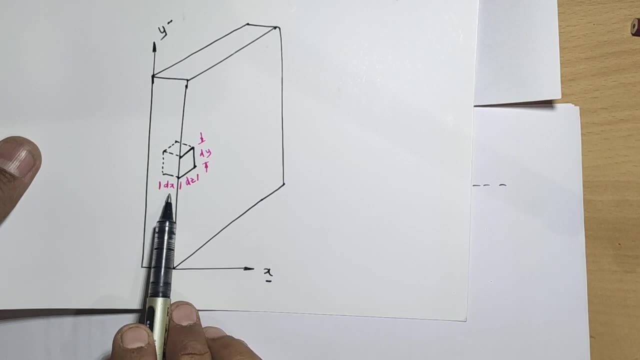 written by taylor series. as we are knowing that the dx is very small element, as i showed in the initial figure, in this particular figure the dx is very small element as dx is small element, so dx square will be again very, very small. and again we are taking 2 factorial, which is divided. 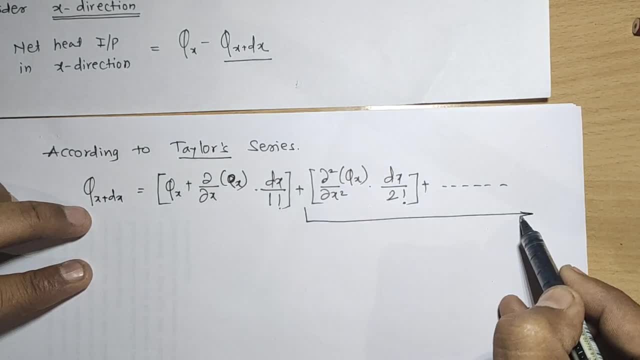 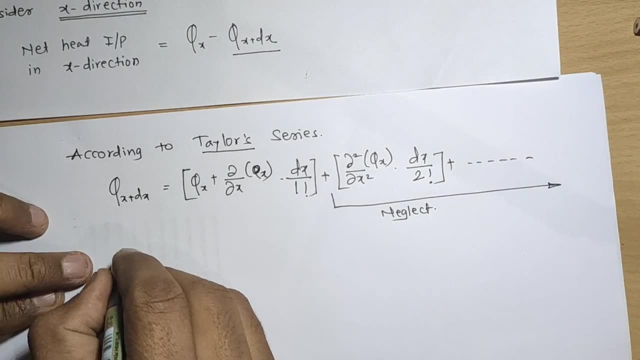 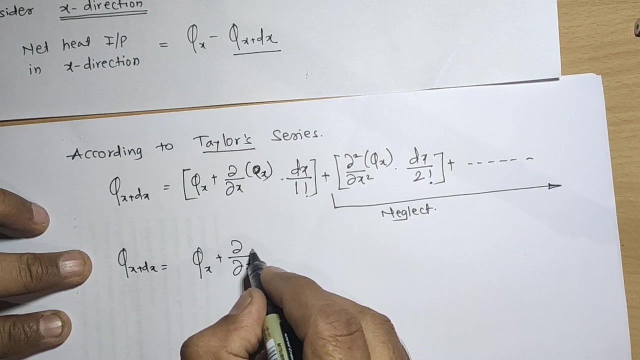 so that will be also very small. so as this term becomes very small here onward, i am going to neglect all other term. so i am going to neglect this one. so now what? i will get: qx plus dx. according to taylor series, it will give you qx plus d of dx. qx into dx: 1 factorial is 1. okay now. 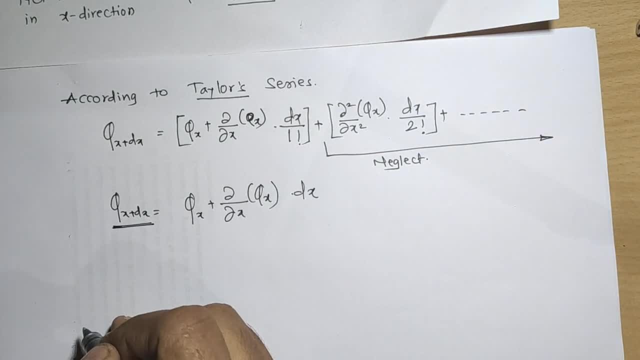 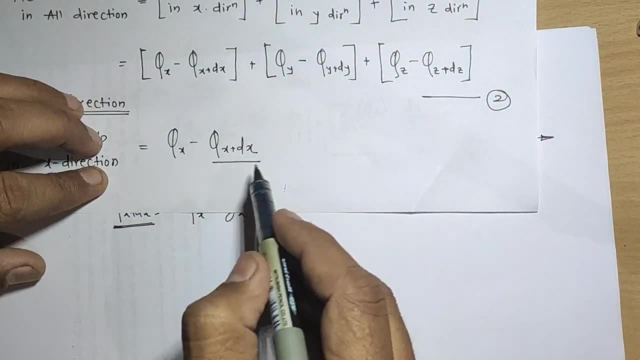 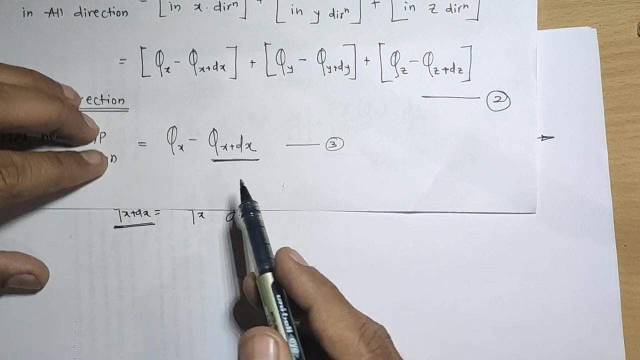 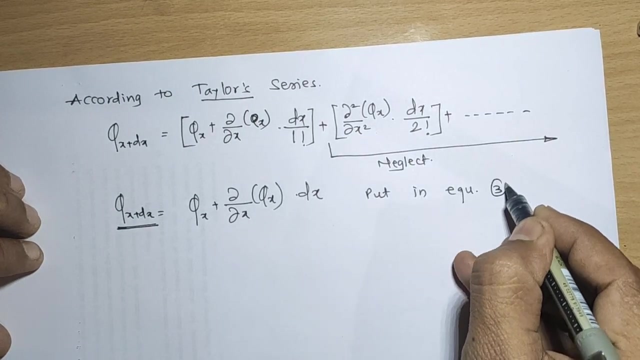 this: we have got qx plus dx. this i am going to put in which equation, this particular equation, that net heat input in x direction is qx minus qx plus dx. so here i am going to write: let's consider this equation number three. so in the equation number three i am going to put qx plus dx equation. so let's put this, put in equation number three. so 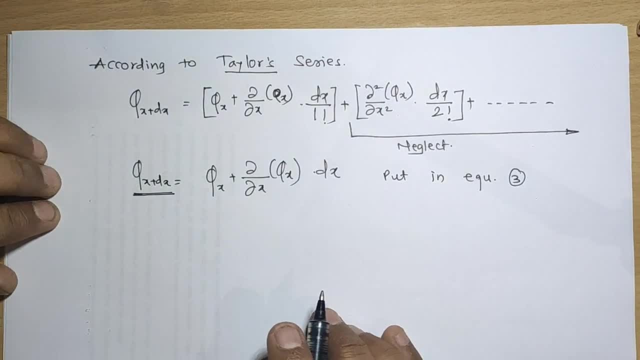 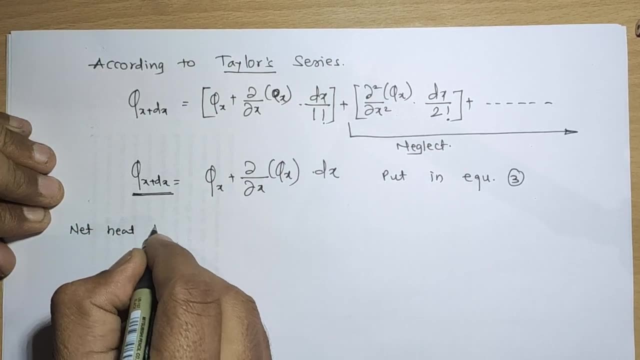 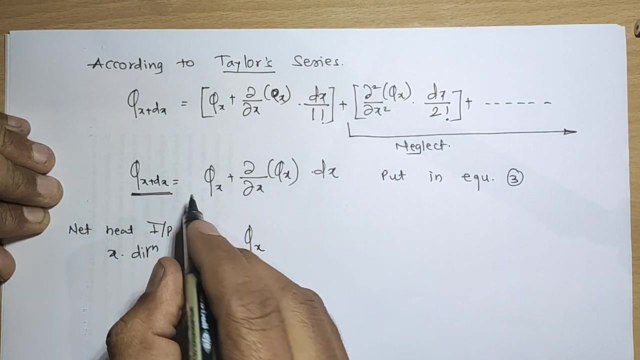 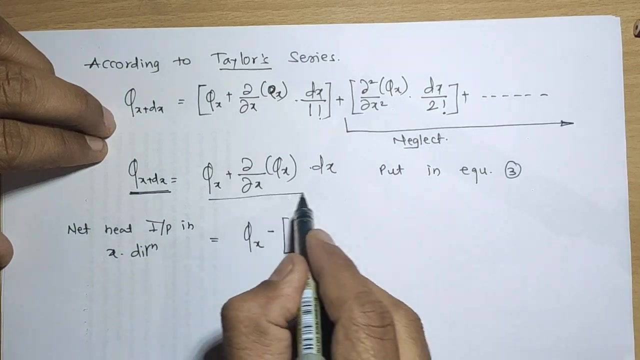 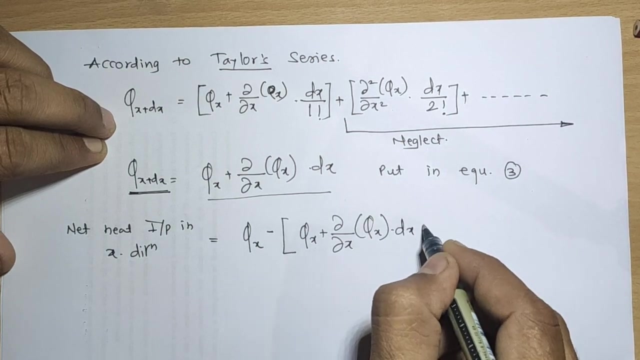 when i put this into equation number three, what we'll get is that net heat input in x direction is equal to qx, is as it is, minus qx plus dx. i have to put it so: minus qx plus dx will become this value i am going to put now. so it will become qx plus daba of a daba, x, qx, d, x. this we 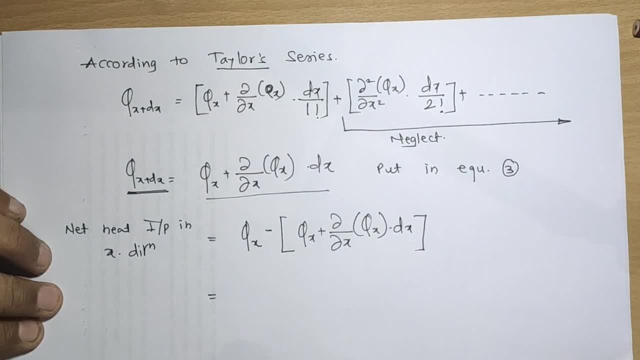 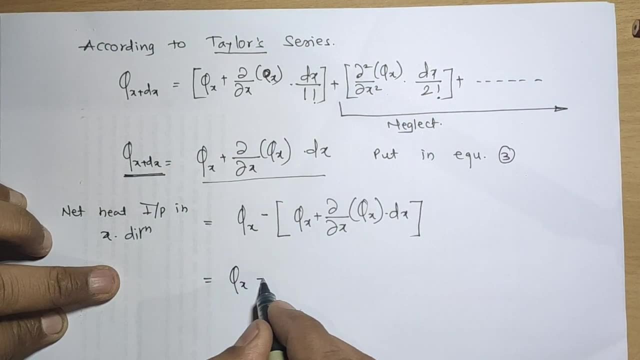 have done it. we have put in equation number two. simplify this particular equation. how to simplify in this particular equation here? what i am going to do is qx. this minus n goes inside, so it will become a qx minus b of dx, qx, dx. that's what equation we have got it. so now this qs, qs will. 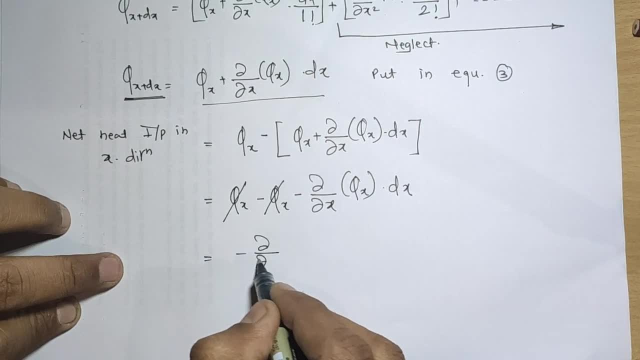 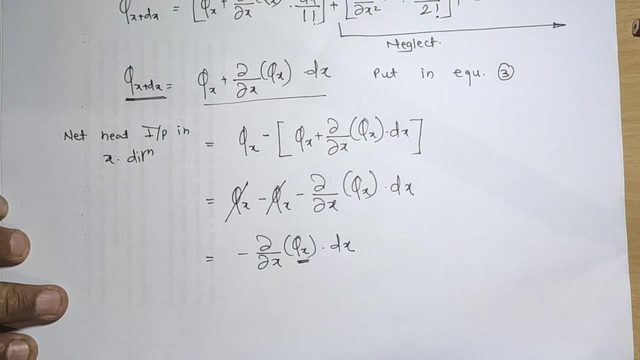 get cancelled. what is remaining is minus d of dx, qx, dx. this is what equation we have got net heat input in x direction. now we know, in this particular, this is what net heat input in x direction, this qx value, this qx value i am going to write according to fourier law of conduction. 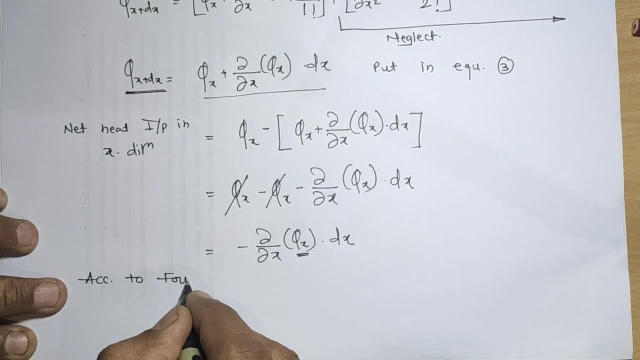 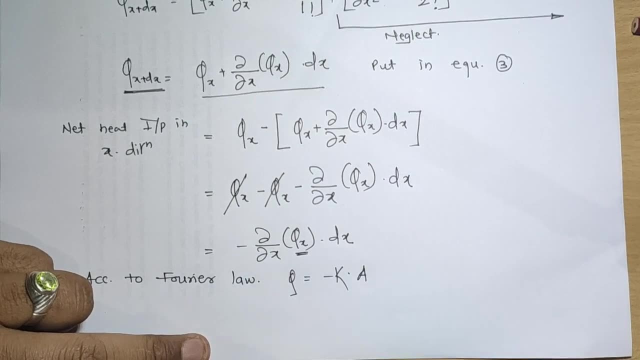 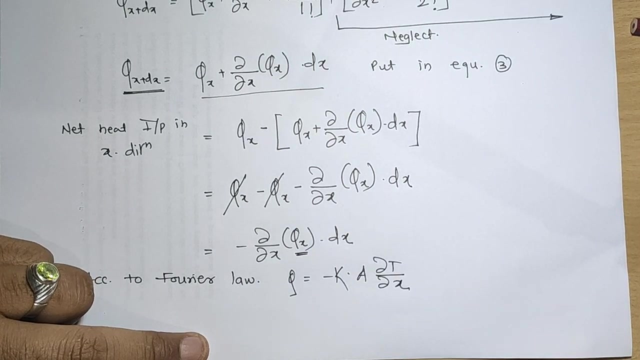 so according to fourier law, according to fourier law, what fourier law says, q is equal to minus k, a dt by dx. so here is partial derivative. so it will be d daba t by daba x. that's the fourier law. so if i am writing this for direction x, so this will become qx. 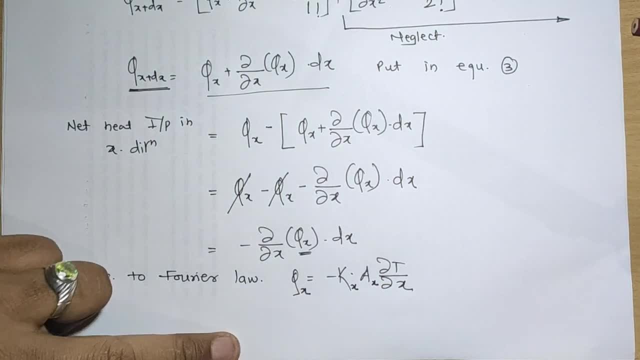 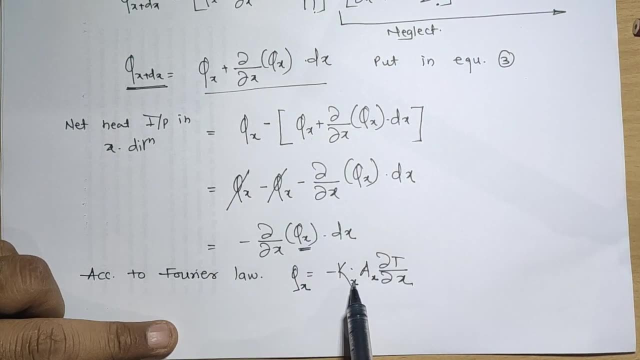 this will become kx. this will become ax if i consider this for x direction. so it will become q x that i have to write here. qx is equal to minus kx. ax divided by div x. what is kx? kx is thermal conductivity in excision. ax is perpendicular- perpendicular. 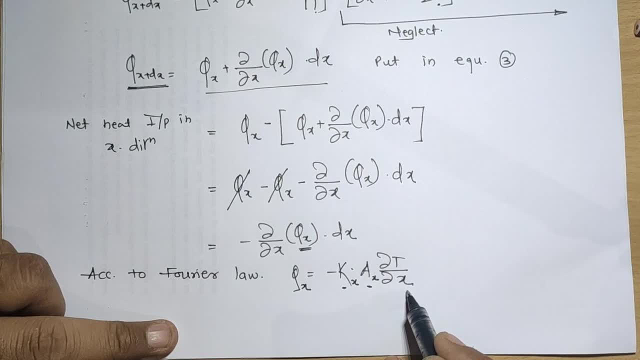 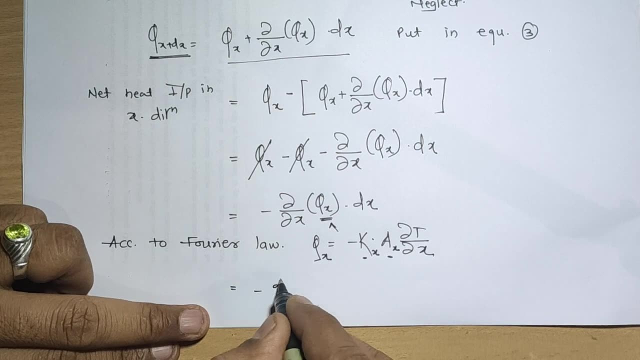 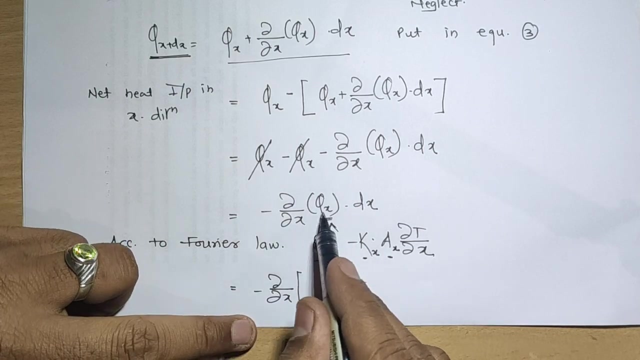 alien x direction. dt by dx is change in temperature with respect to x. so this i am going to put here. so what will get an heat equation? now the equation will become minus diaba by daba x into bracket, into bracket, this term. this term means what minus? 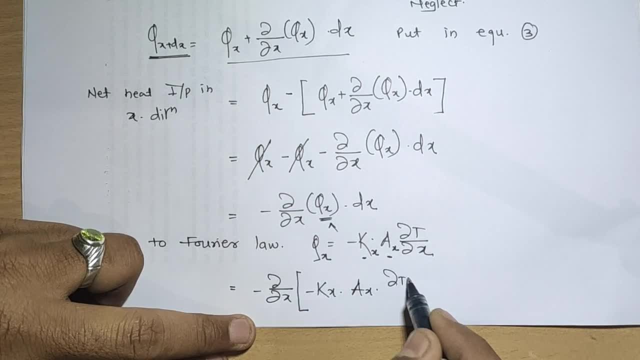 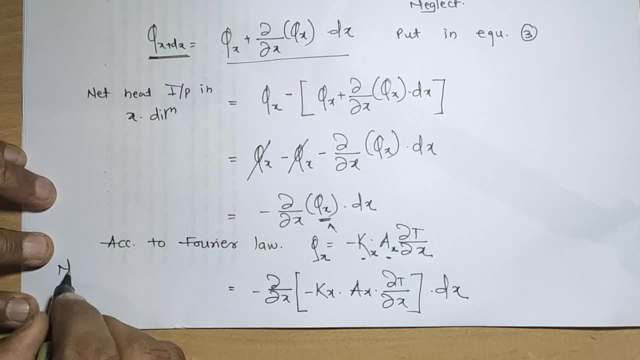 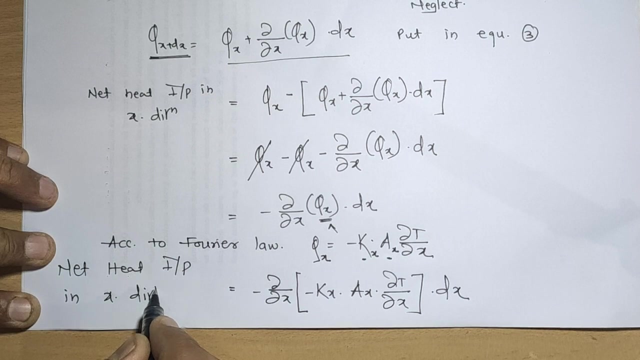 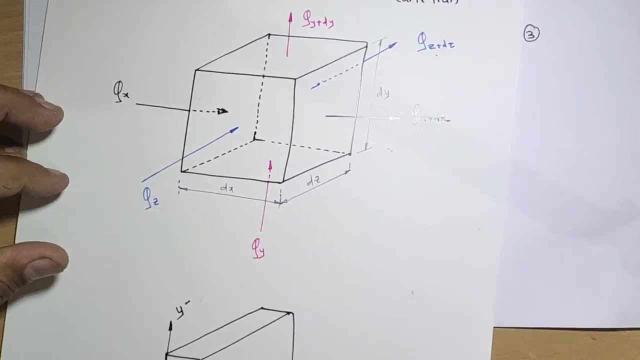 minus kx, ax, daba t by daba x into dx. this is what we have got, an equation for what heat input, net heat input in x direction. now i am going to simplify this: what is the ax that we have to see? ax is what area perpendicular to x direction? what is the area perpendicular to x direction? 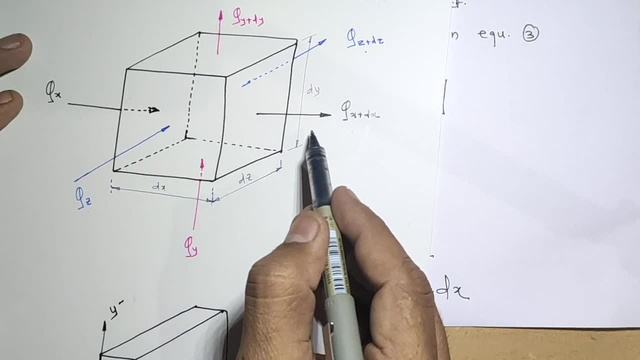 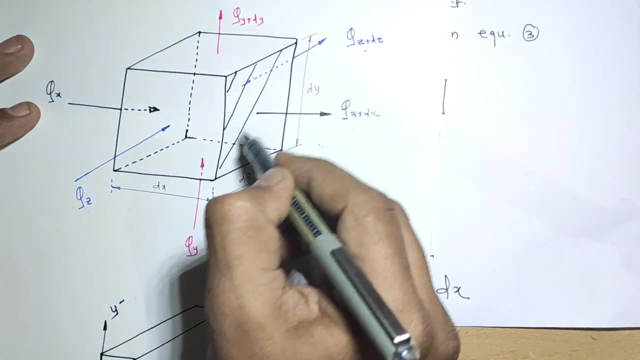 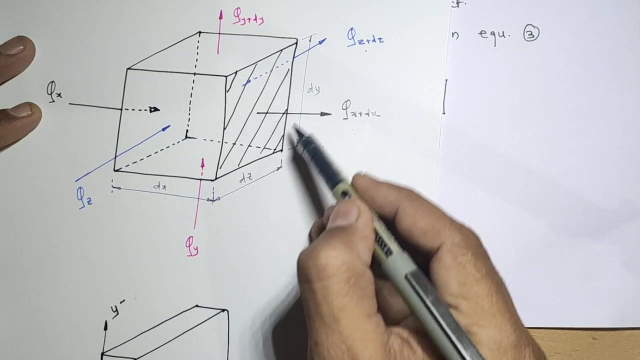 this is the x direction. if i consider this is x direction, then what is perpendicular area? perpendicular area is this one. the perpendicular area is this perpendicular area. so what is dimension of this, this perpendicular area? dimension of this perpendicular area is what dx and dy this will give you this particular area. okay, so, rather than ax now, 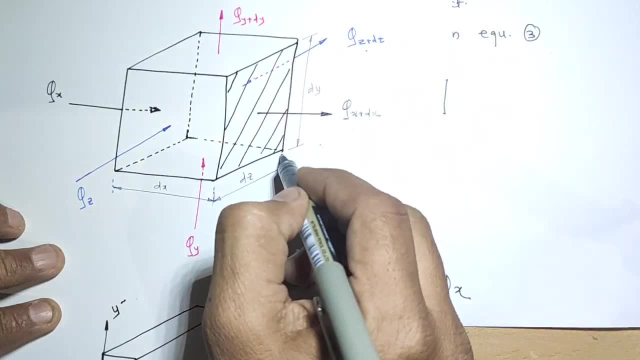 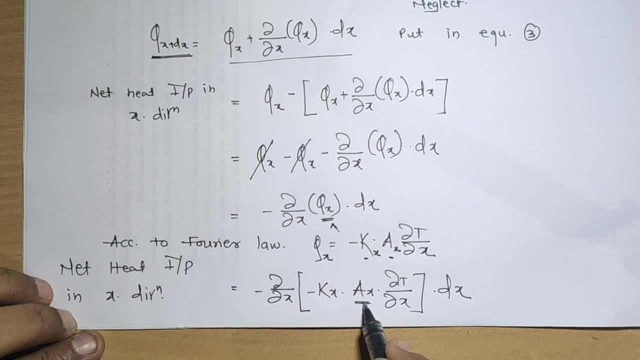 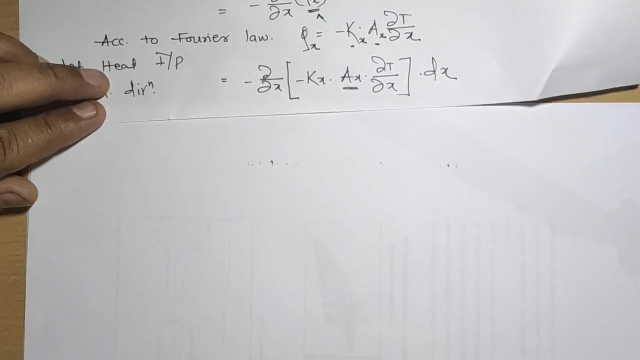 ax. what i am going to write is dy into dz or dz into dy. this i am going to put okay. so in this particular equation, i am going to replace ax by using dy. so let's write this particular equation now. net heat input in x direction. net heat input in x. 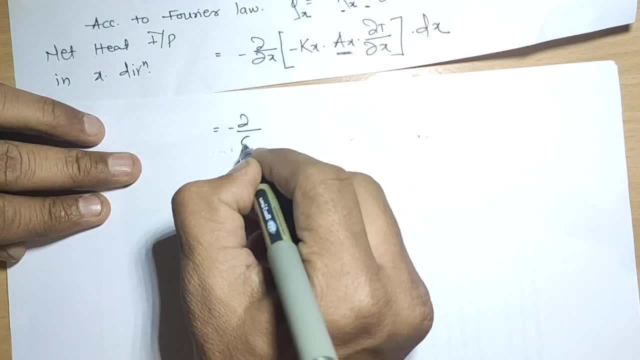 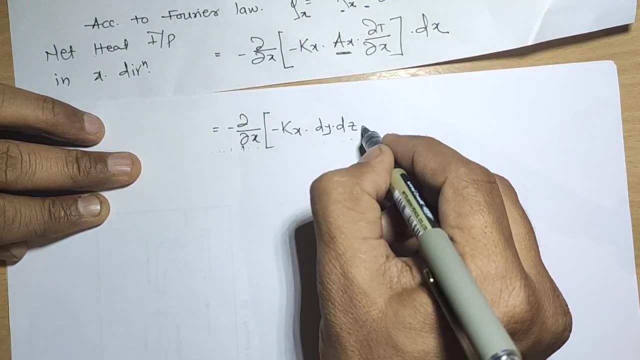 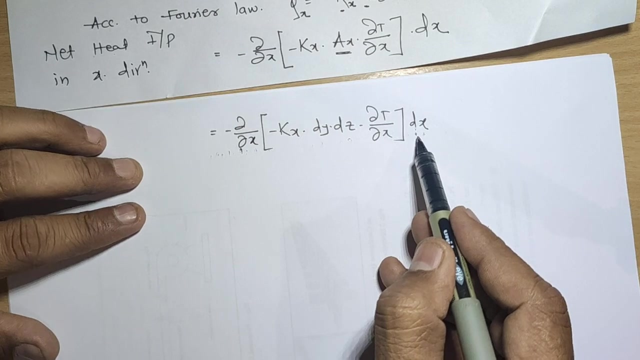 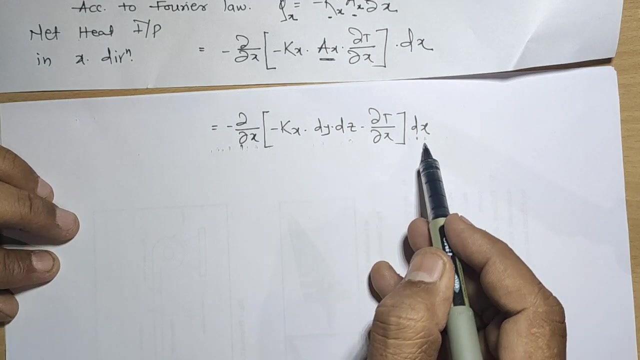 direction will become daba by daba x into bracket minus kx, ax. i am going to write d y, d z, daba t by daba x, dx. you have to understood here: dx is complete derivative and daba is what. daba is what partial derivative dx. some of the time it is also called as exact derivative and daba is. 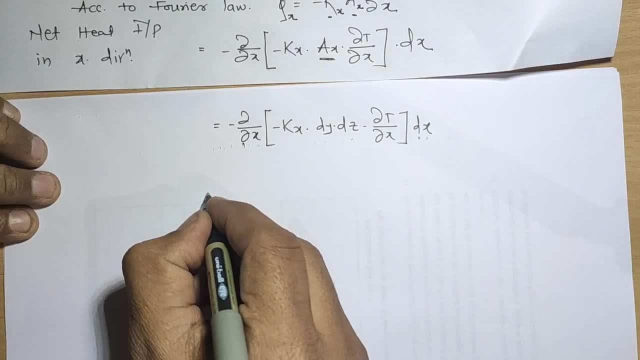 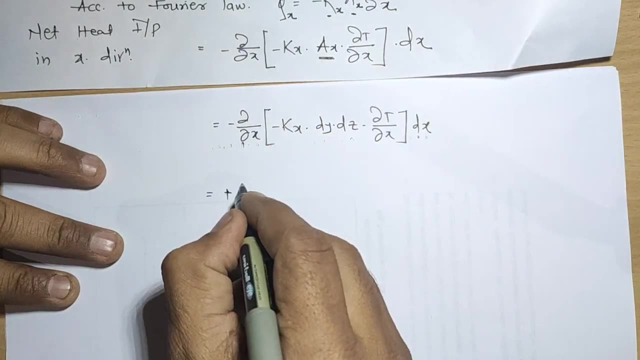 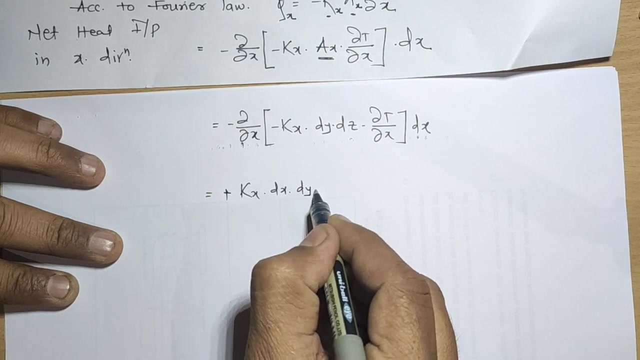 called as partial derivative. okay, so again, simplify this particular equation. how to simplify this? this i will take inside, so minus, minus will become a plus, so plus i will write kx. this d x comes on inside, so it will become a d x, d y, d z. what i done, this d x i have put here and this: 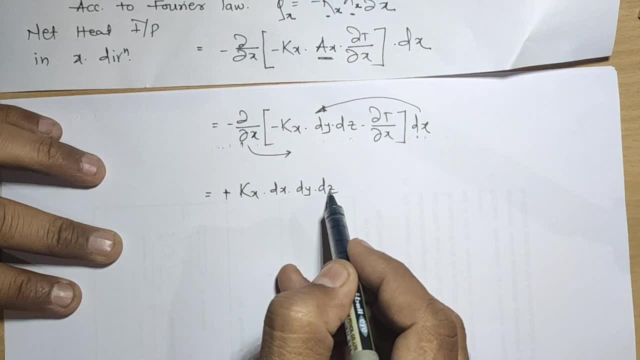 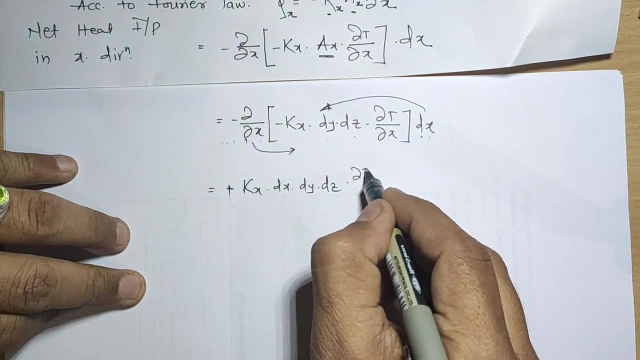 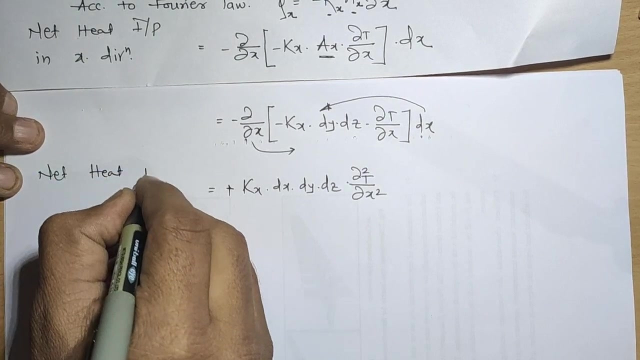 i have taken inside, so it has become a k x d x, d y d z, d x, d y d z into this and this: it will become a square, daba square t by daba x square. this is what we have got: net heat input in x. 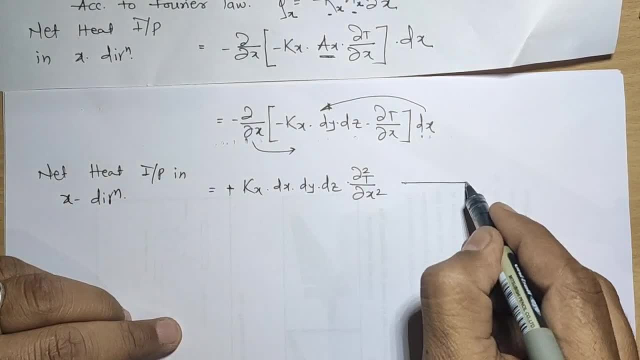 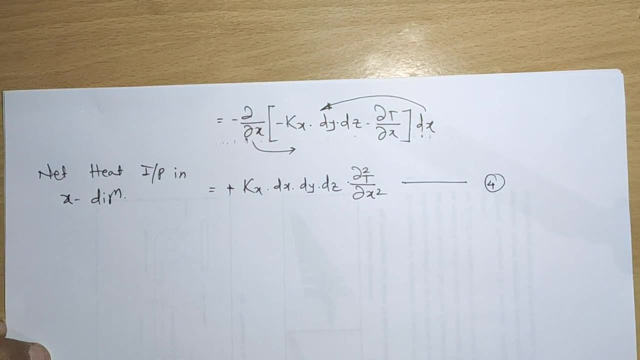 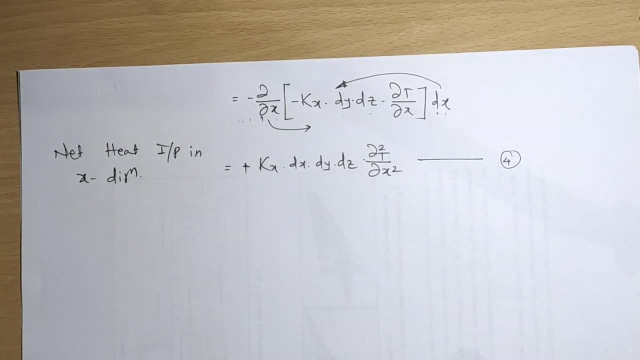 direction. so we have got this in x direction. that's the equation number. if i check, if i go back and if i check the equation, this is the equation number four. so we have got equation for equation number four. now what i have to do similarly, i can write here similarly. 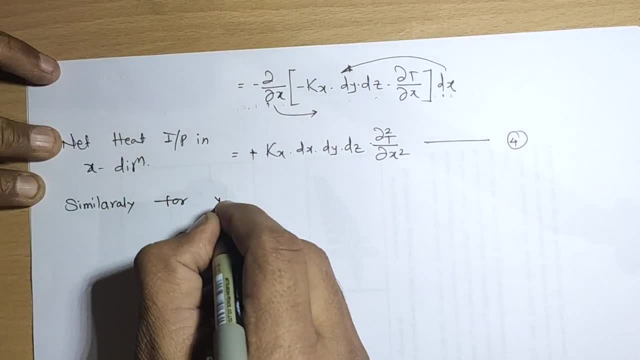 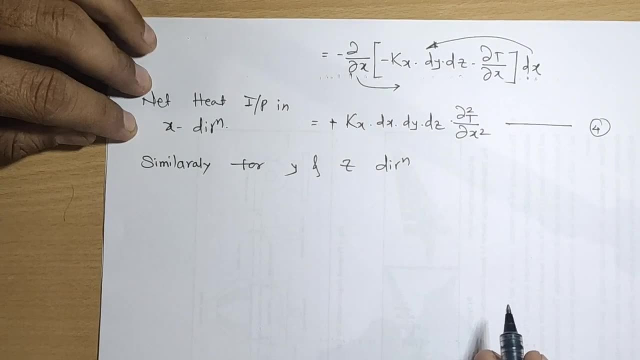 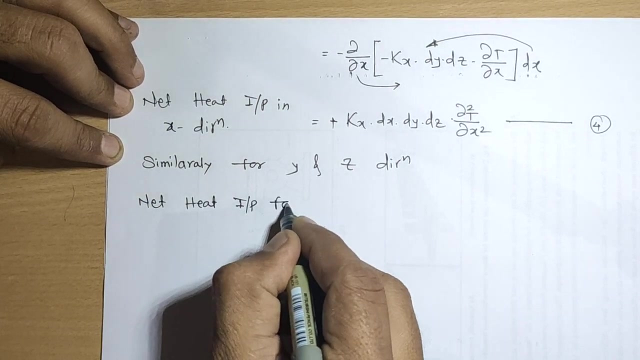 so we will get equation directly y and z corresponding to연 s in y and z direction, withguning these into y and z. so in that i can 내려 use this equation in the form of a square and getting the complete common portion of the equation, that is, y and z. 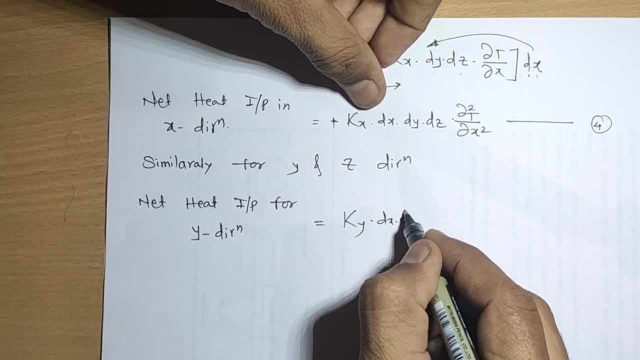 so this equation of monitor in this equation is what my equation is going to take. so i am the teacher of the equation, is accordingly who i am. and then i'm going to 60 Dx, Dx, Dz for y and z direction. we can get this equation number four for y- z directions. so what will get y and z direction? similarly, net heat in p stuck for y direction also gets correctal energy for y direction system toasts, the general frequency and forecasting density着. 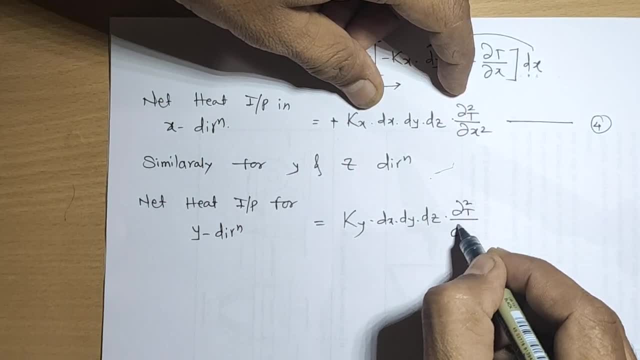 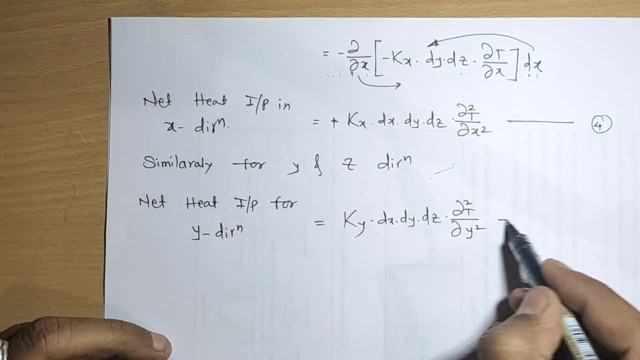 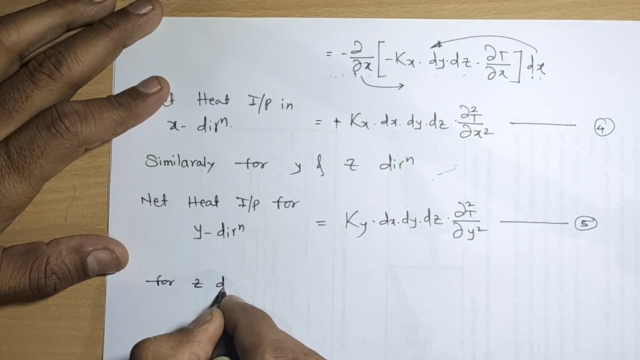 instead of this, it will become a daba square, t daba y square. so what is the change here? instead of x, i return y. instead of x square, i return y square. that's the equation number five. similarly, net hit input for z direction. so what will be equation for z direction? equation for z direction. 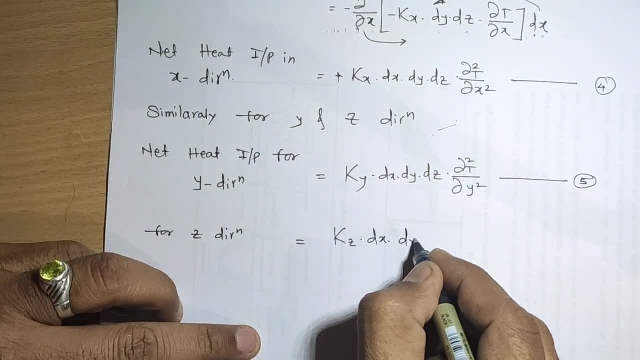 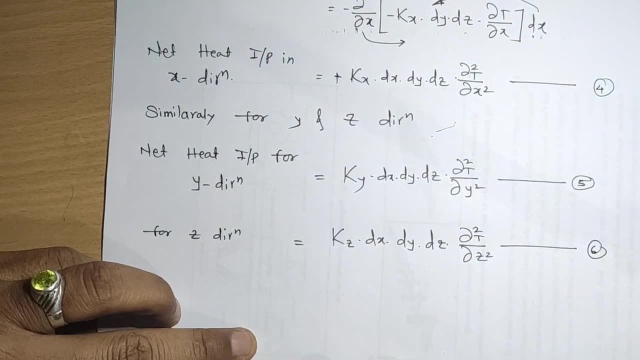 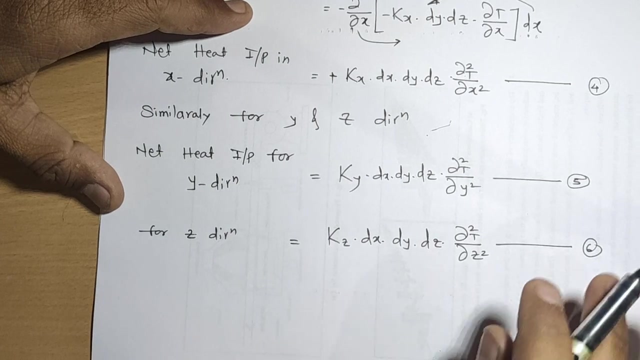 will become a kz, dx, dy, dz daba square, t daba z square. so we have got net hit input for three direction. that is x direction, is equation number four. this is x direction, this is y direction, this is z. now total hit input will be summation of all this. total hit input will be summation of: 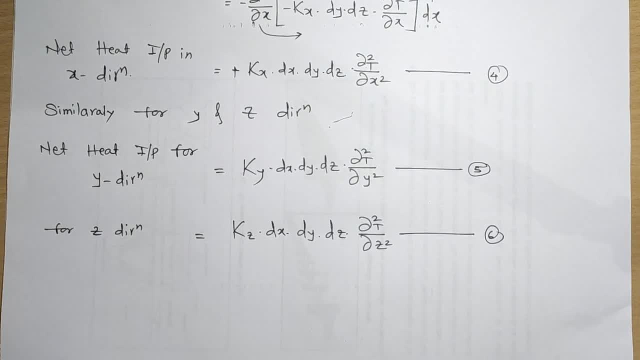 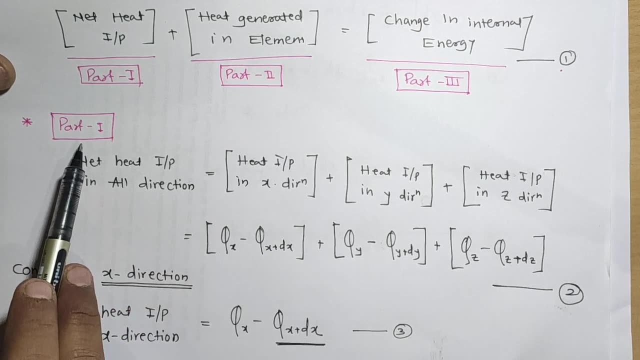 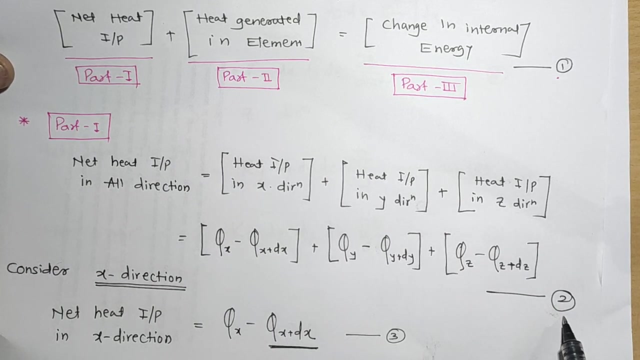 all this. so in the initial equation we have written, referring to this particular equation, in this particular equation, net hit input. that is the part one. part one is what hit input in x direction, y direction, z direction. so from that we have written equation number two. in equation number two i am going to put value of this, this and this by using equation number four. 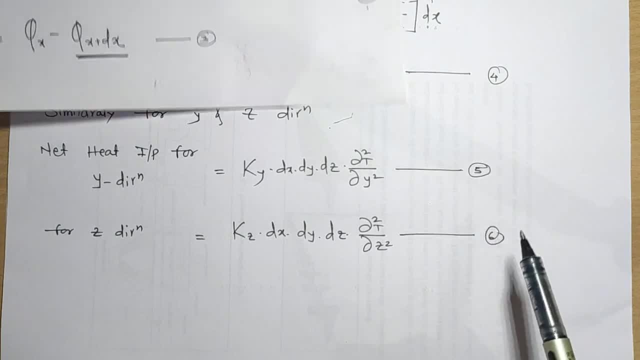 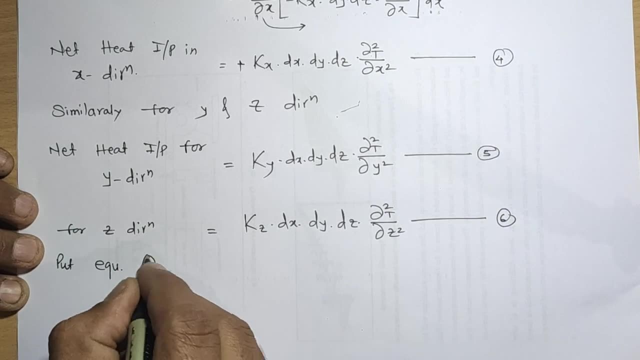 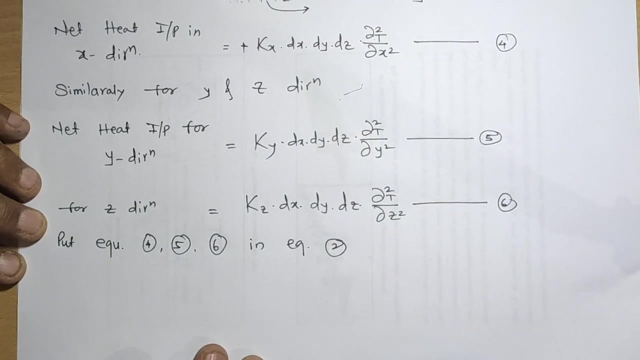 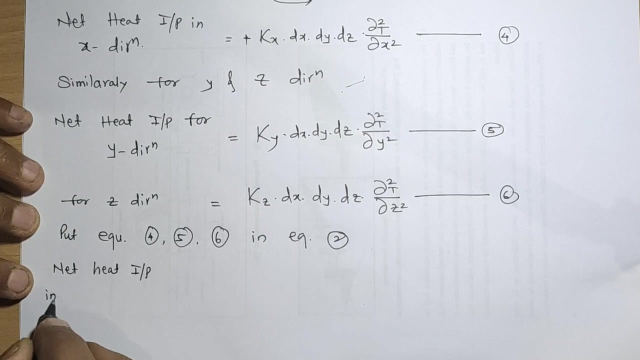 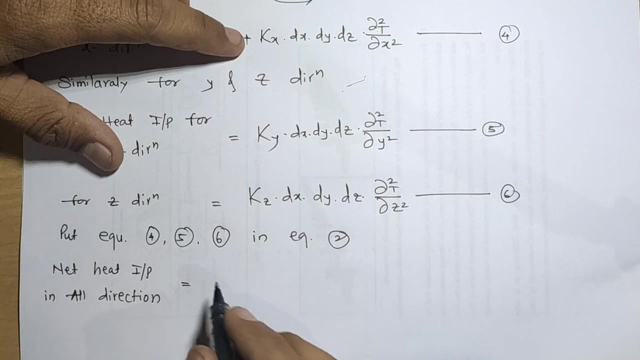 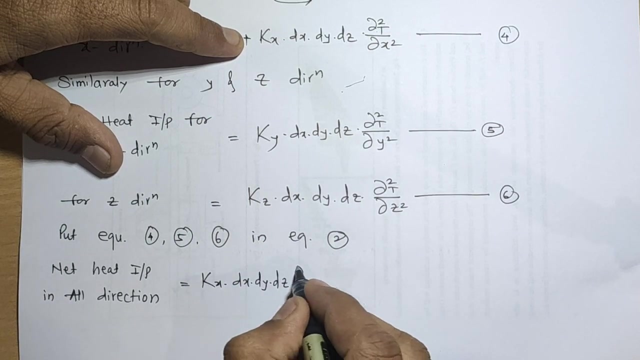 five, six. so i will put equation number four, five, six in equation number two. okay, so put equation number four, five, six in equation two. so what will get an equation? now, net hit input in all direction, in all direction i will get as equation number four. what says equation number four? kx, dx, dy, dz, daba, square t. 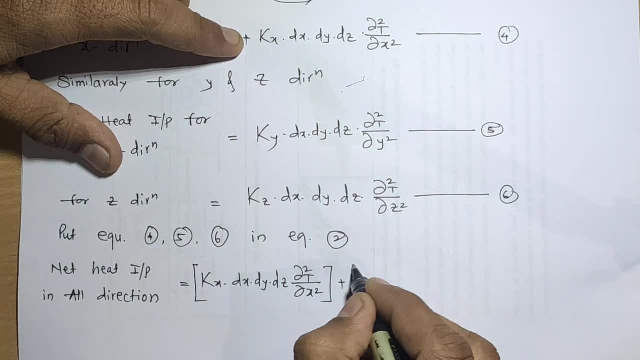 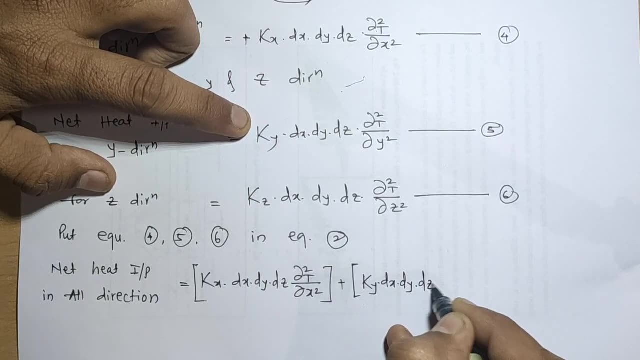 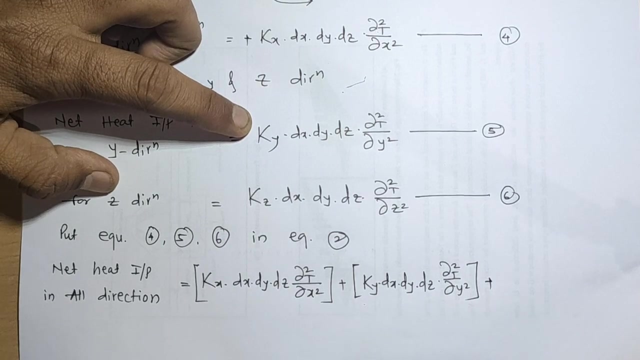 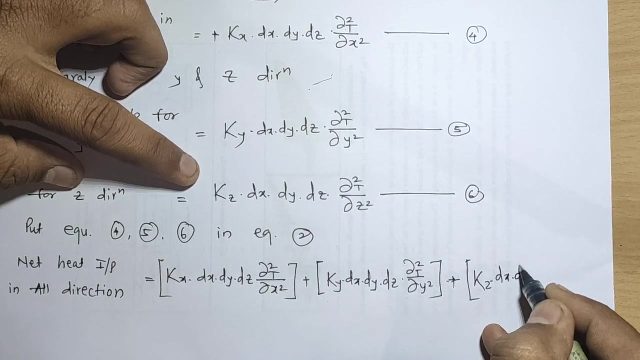 daba x square, that's in x direction plus in y direction. what it says. equation number five: k y, d, x, d, y, d z into daba square. t daba y square, that's the in in y direction plus in z direction. in z direction is this one so k z, d, x, d y d z daba square. 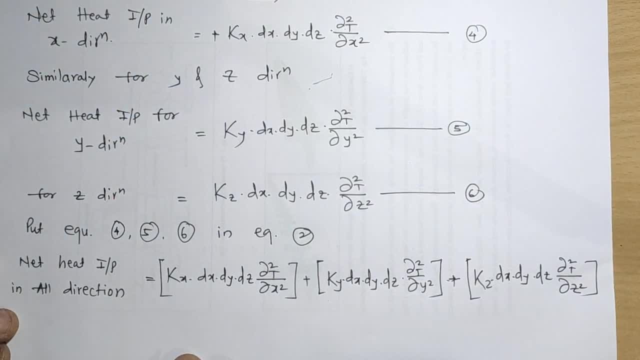 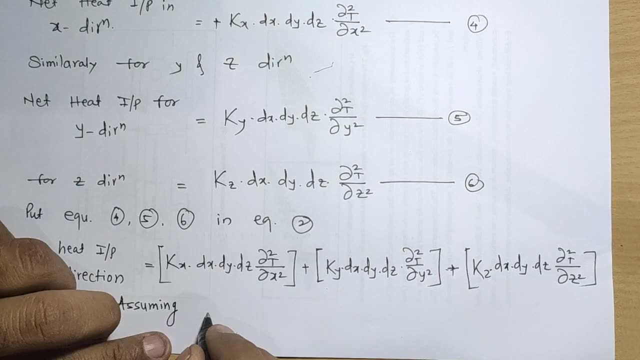 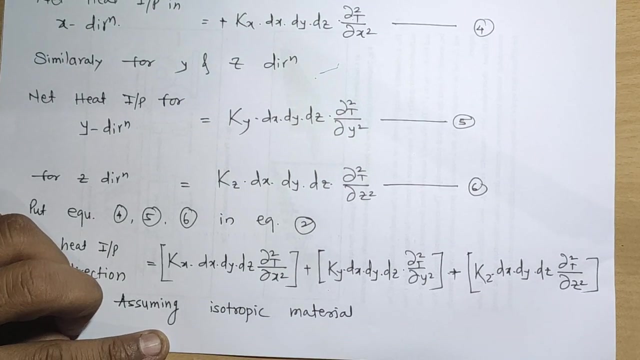 t daba z square. so we have written for three simplifying this particular equation. how to simplify, assuming for the isotropic material. isotropic material is what material which has the same property in all direction. so i am assuming that is isotropic material, so property will be same. 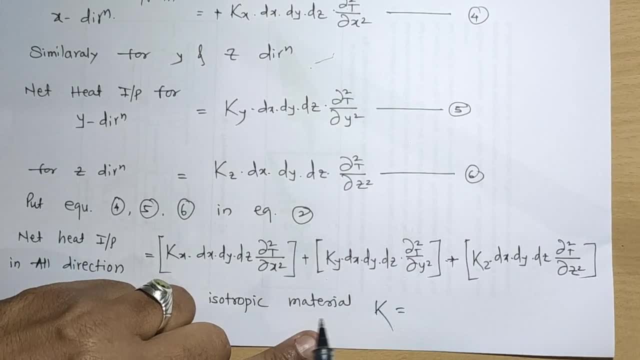 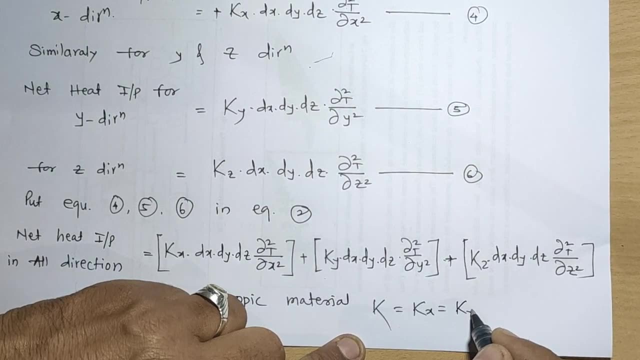 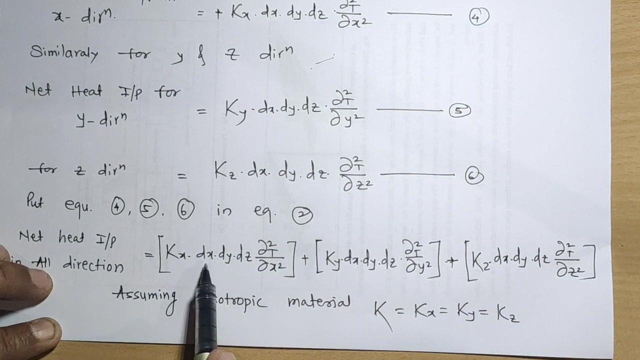 in all three direction. so what i am going to assume is thermal conductivity in x direction, y direction, z direction is same, so it will become: k is equal to kx is equal to ky is equal to kz. so i consider kx, ky, kz is same, so from this i can take common k at the same time: dx, dy, dz. so what? 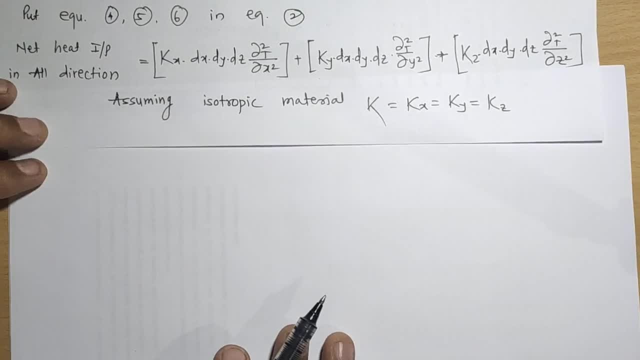 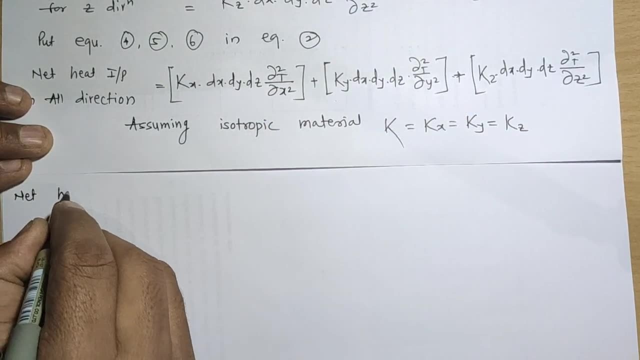 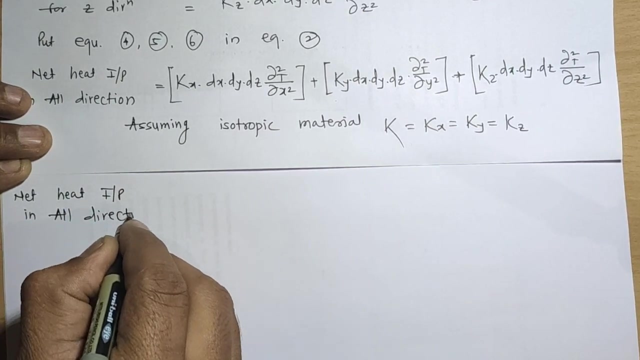 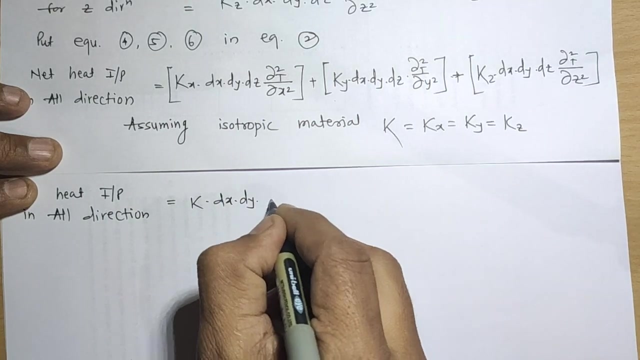 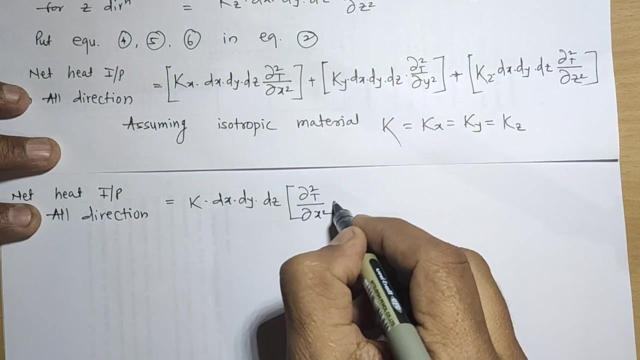 our next equation will get. the next equation is like this: in this particular equation, let heat input in all direction, in all direction is equal to. i am going to take common k and dx dy dz, so k you, dx dy dz, into bracket. what it remains, it remains this term: daba square t, daba x, square plus daba. 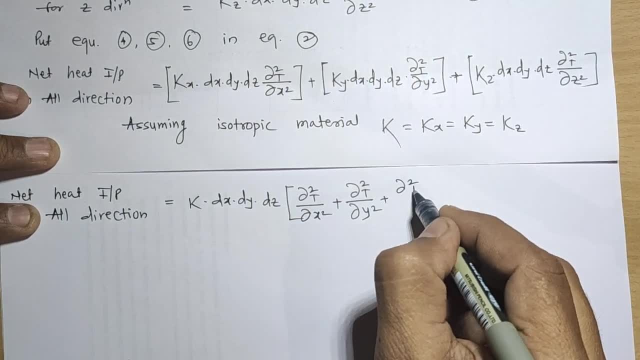 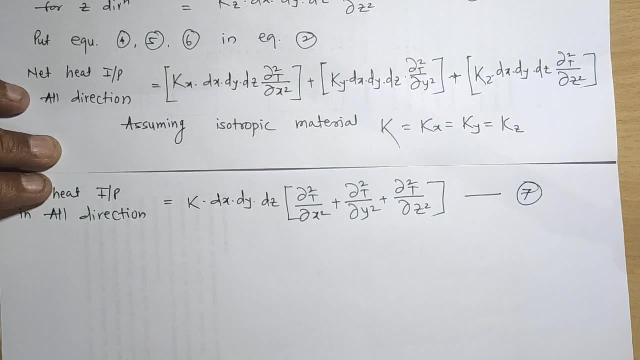 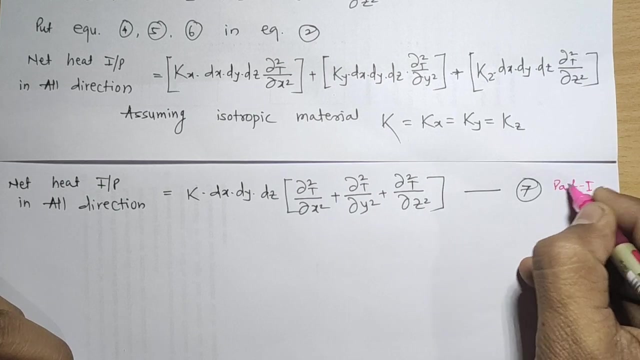 square, t daba y square, plus daba square, t daba z square. so we have taken common this and this will be equation number seven. this will be equation number seven and this will be equation for our part number one. so part number one gets completed here. okay, so this is part number one. now i have to. 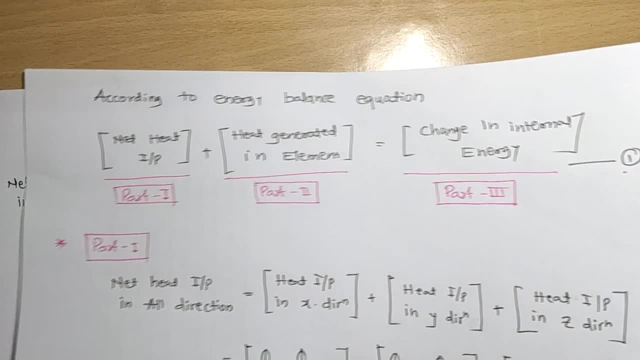 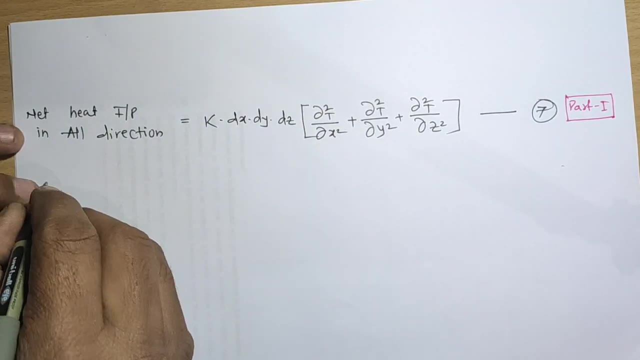 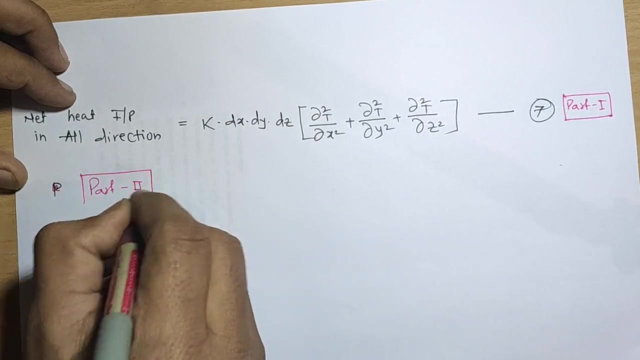 go for part number two. what is the part number two? if you refer this vertical figure? part number two is heat generated in the element. okay, so let's consider now part number two. now i will consider that the part two. so what gives a part number two? part number two is heat generated in the element. 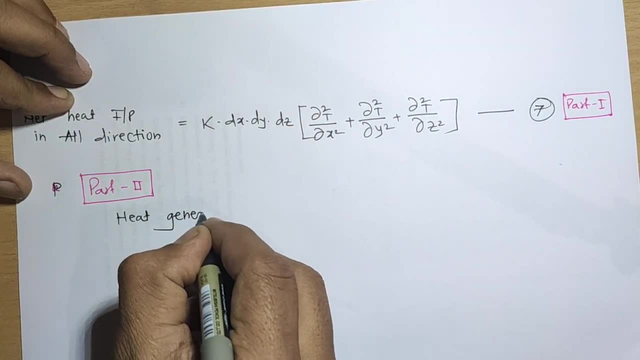 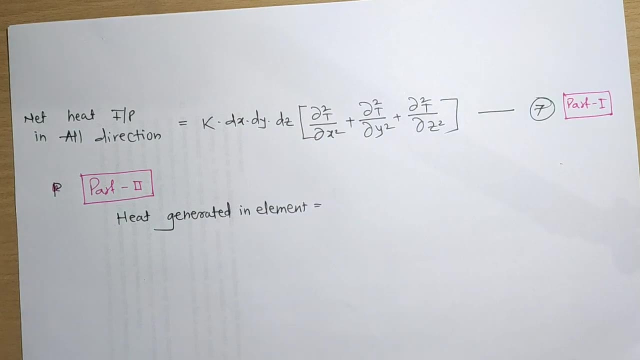 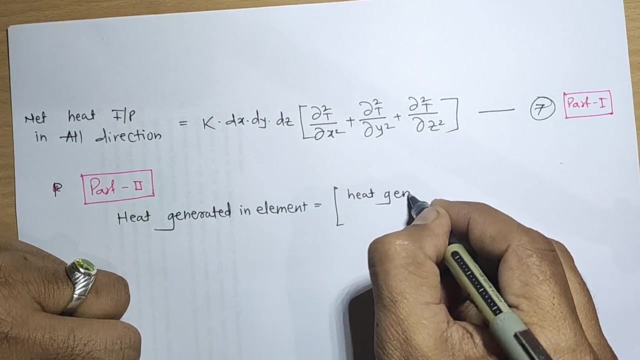 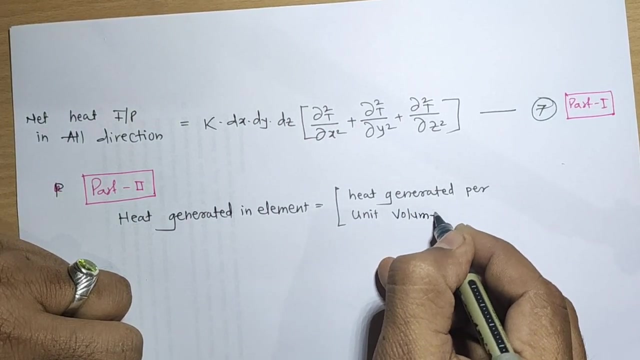 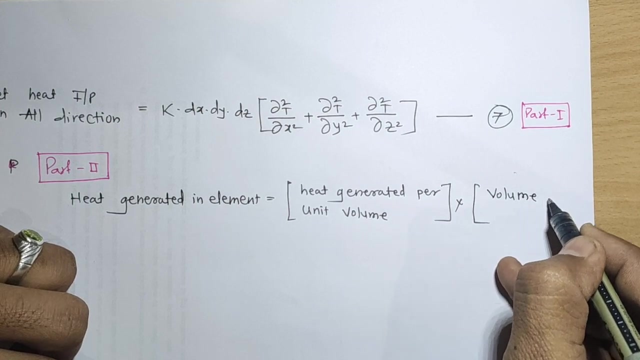 heat. the heat generated in element is nothing, but this is generated. i can write one thing: that heat generated, heat generated per unit volume into volume of element, into volume of element, into volume of element. that's the equation for net heat generated. why? because this is the heat. 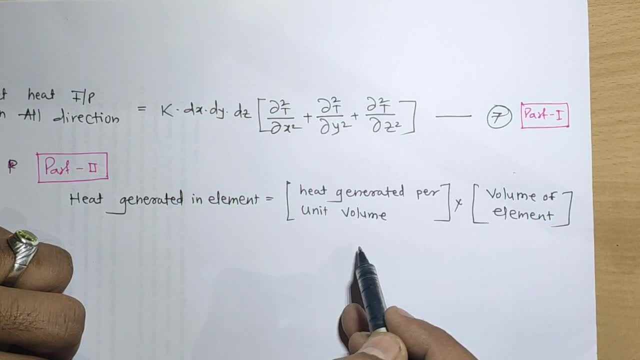 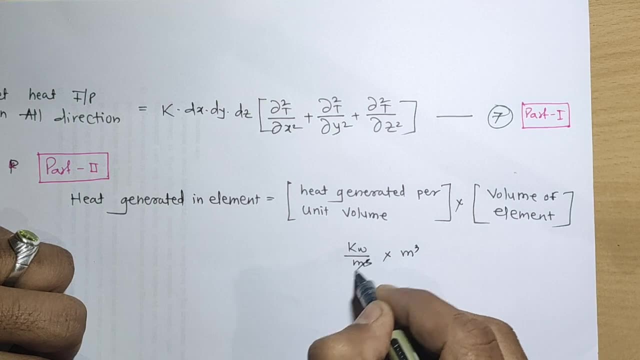 generated per unit volume that we denote by small qg. if it is per unit volume, so its unit will be what kilowatt per meter cube? and if i multiply by meter cube, the meter cube, meter cube get cancelled, it will get a kilowatt. so we want a net heat input. so that's why we are going to write this one. so 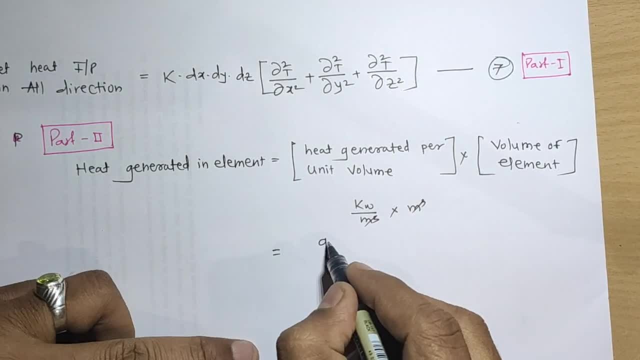 net heat input is generally denoted by qg, which is having unit as heat transfer per unit volume into volume. now what we are going to do is we are going to write this one. so net heat input is supposed to be the unit heat that is producing the C, p and n. ifk would be held at does not mean that 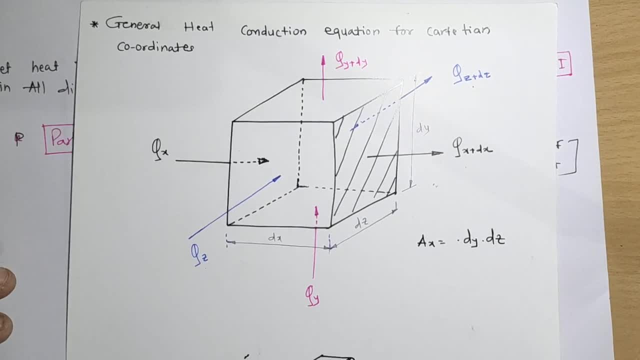 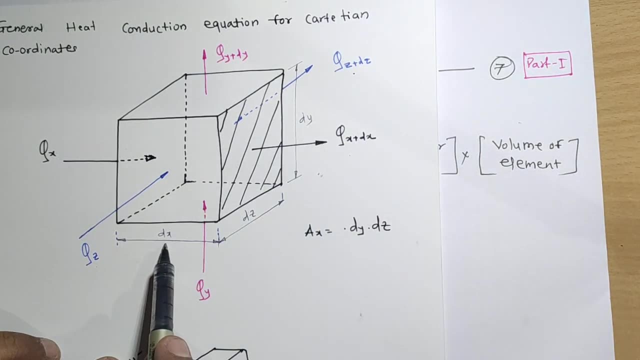 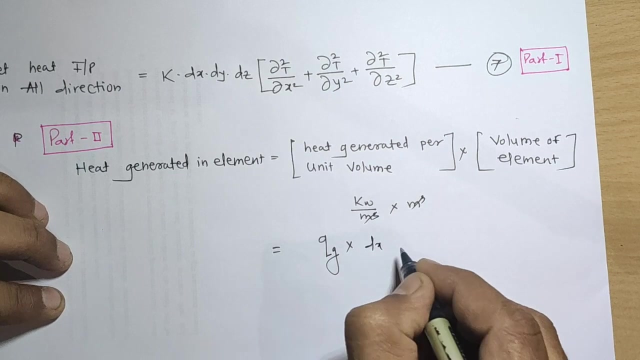 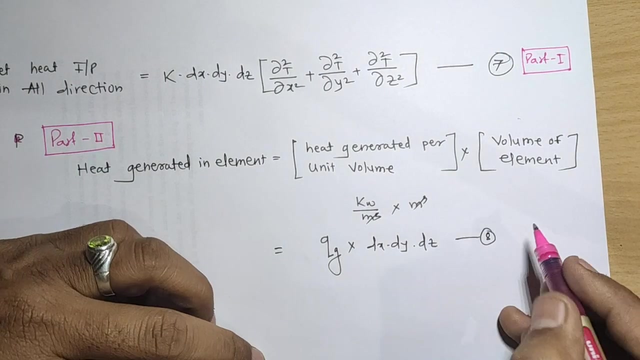 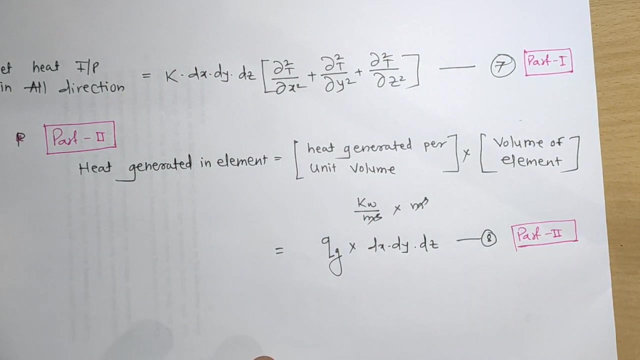 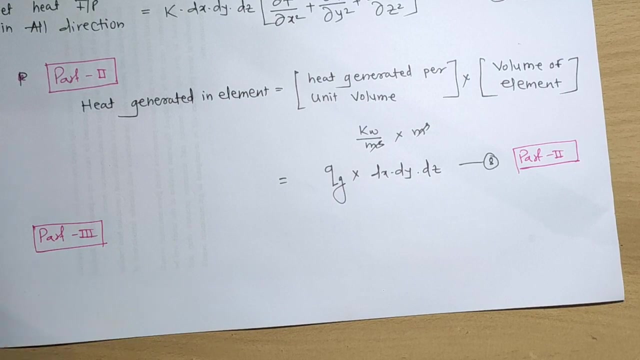 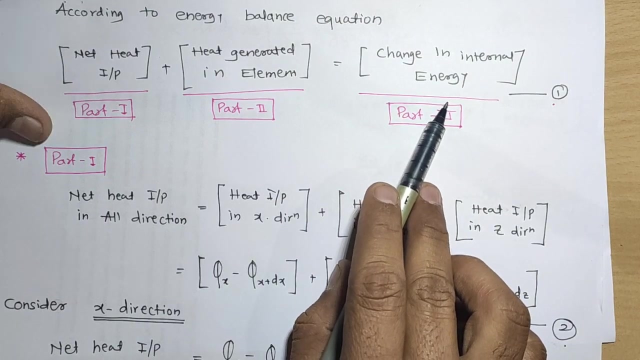 energy as per引thing any others. two is quite easier one. now let's go for part number three. part number three: what is our part number three if you go for basic equation once again here in the basic equation, change in internal energy. part number three is: what change in internal energy? so let's consider: 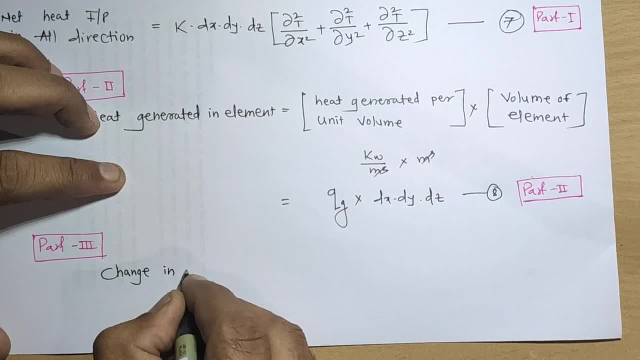 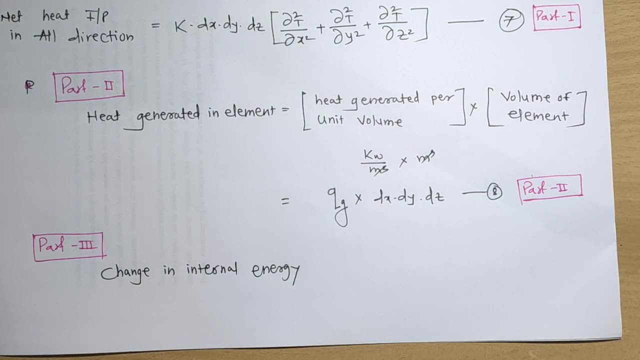 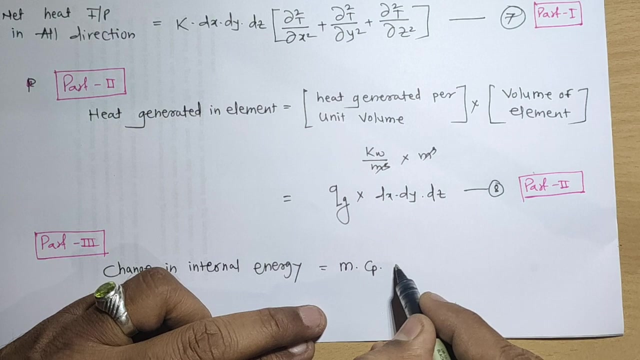 change in internal energy. and this change in internal energy, i'm going to use a simple equation which says mcp delta t. so this i'm going to write mcp delta t, delta d, change in temperature. but here it's unsteady state, so i'm going to write change in temperature. 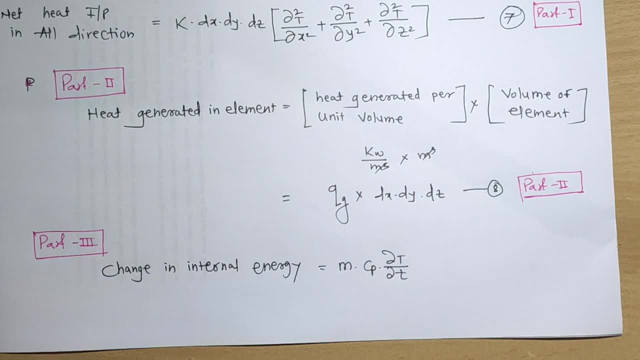 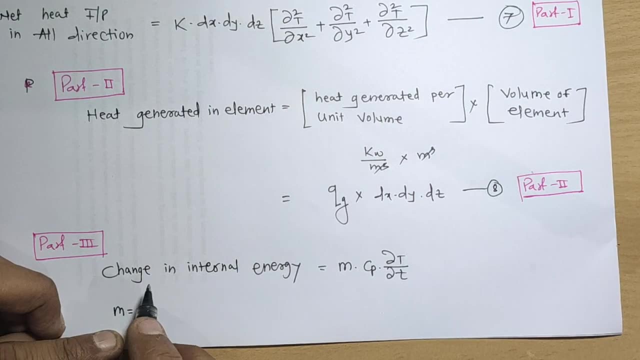 with respect to time, the dot, t by dot. i have written it okay. so this is change in internal energy, part number three. in this case, i can write that mass is nothing but mass is nothing but density into volume. this is standard equation, how we can write, because mass may have unit. 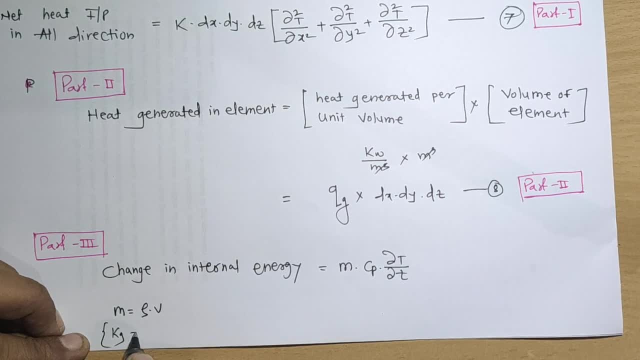 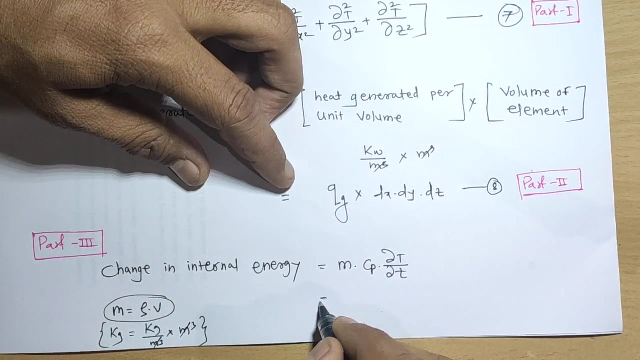 as kg. mass may have unit as kg. so this i am writing a unit: density is kg per meter cube. what is volume? volume is meter cube, so meter cube, meter cube get cancelled and we'll get kg. so mass can be replaced as rho v. so this equation, what i am going to write is rho density. 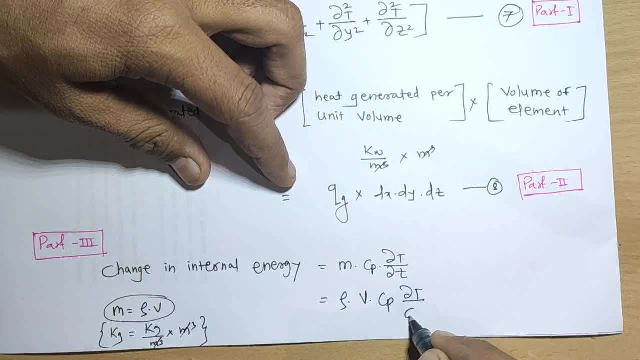 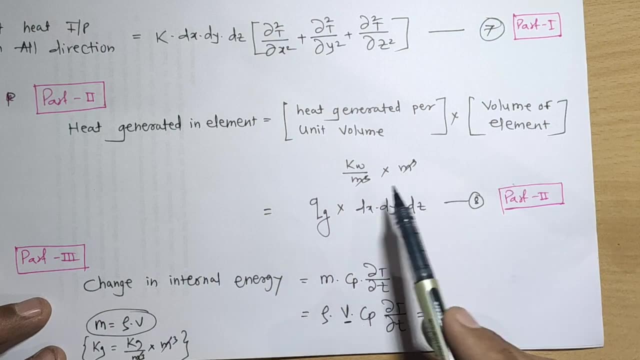 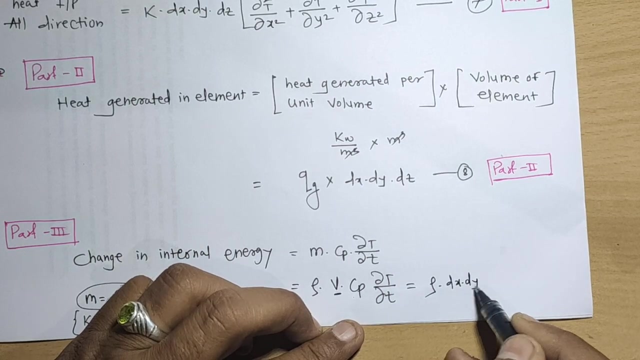 into volume, into cp other term as it is, dot t by dot t. what is the volume? that you are knowing? what is the volume just now? we have written here that volume is equal to volume of element. is what? dx dy dz? same thing i am going to write here. so rho into dx dy dz and 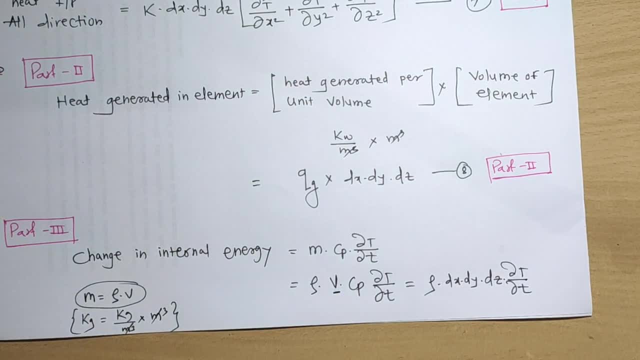 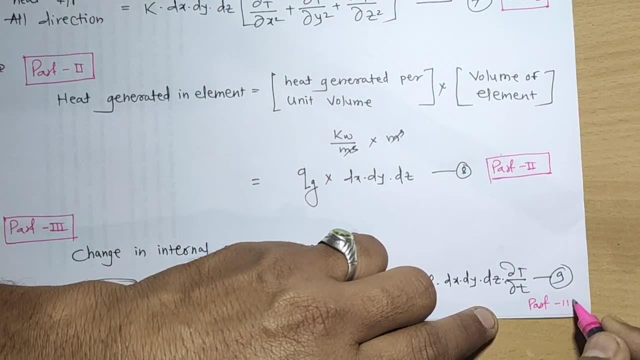 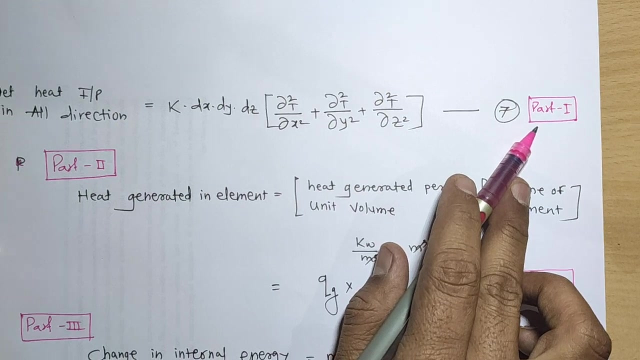 then dot t by dot t. this will give you equation number nine and equation for part number three. so we have got equation for all three parts. now, here we have written part number one. part number one, which is nothing but net heat input and net heat input. we have got this equation part number two, which is heat generated in. 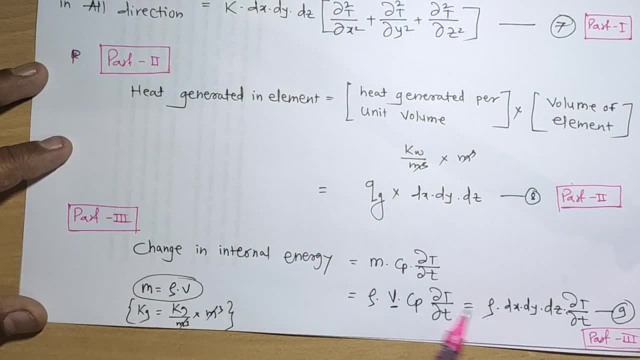 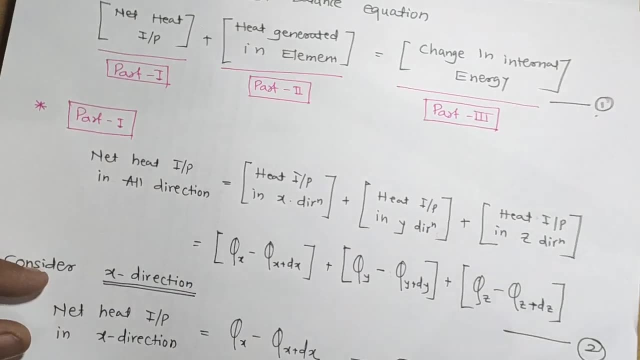 the element. we have got this equation and part number three, which is change in internal energy. we have got this particular as a equation, now all three part. we have got now all three part. i have to put in equation number one, which is our basic equation. that is part one. 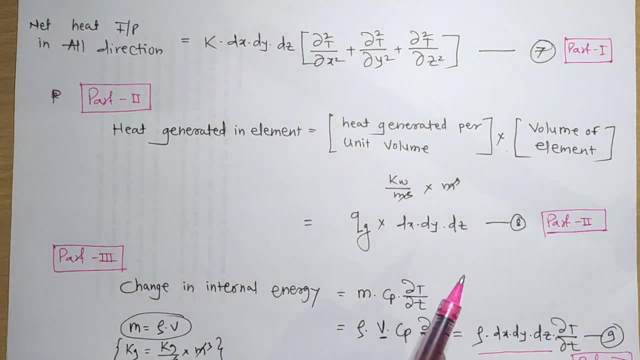 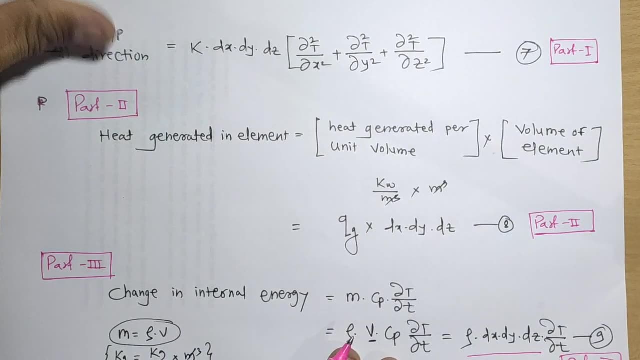 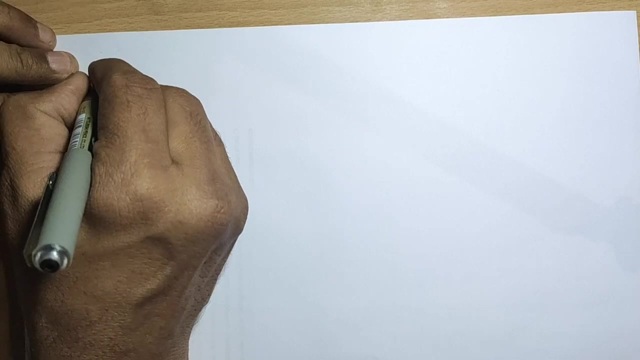 part two, part three. so in equation number one i am going to put equation number seven, eight and equation number nine. so now let's put this: all these three parts i am going to put in equation number one. so i will write here as put: equation number seven, eight and. 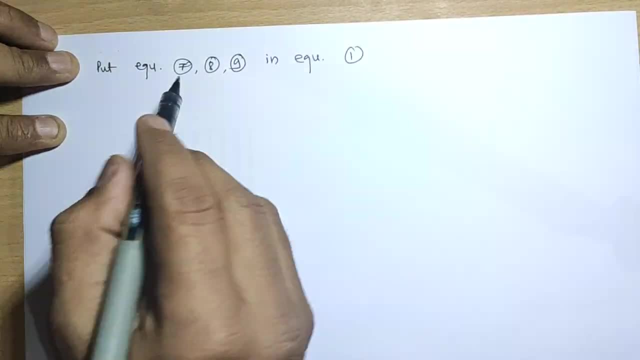 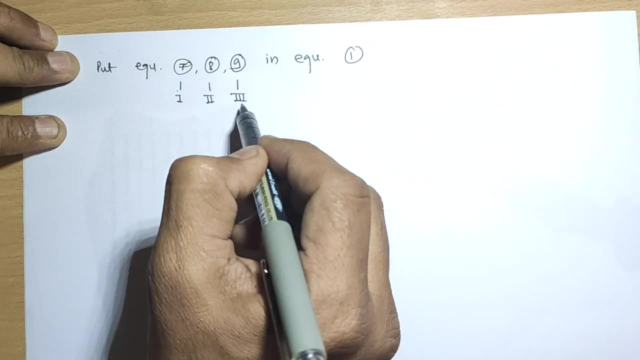 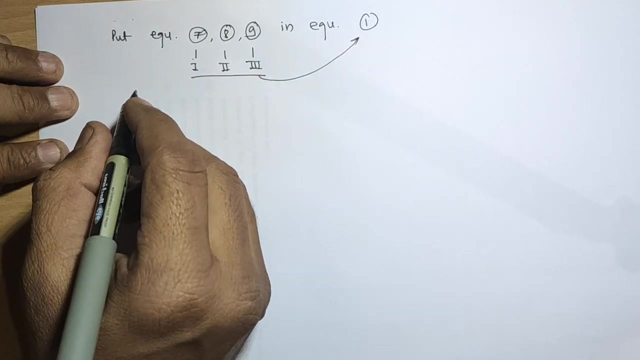 nine in equation number one. so equation number seven is part number one. equation number eight is part number two. equation number nine is part number three. these three i am going to put in equation number one. so what? we will get it the part number one. what is part number? 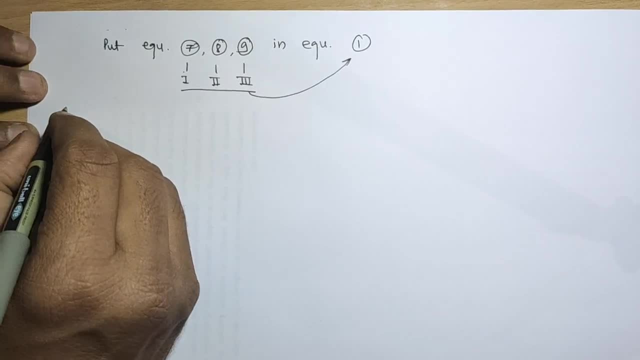 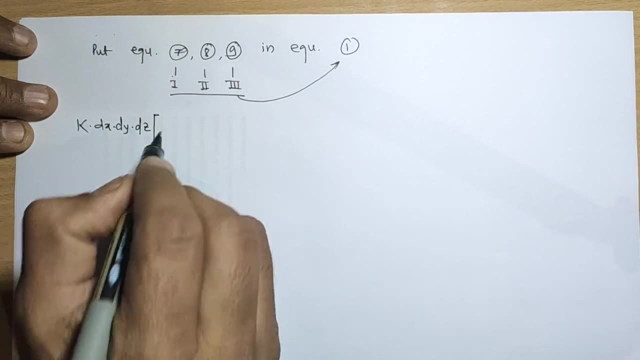 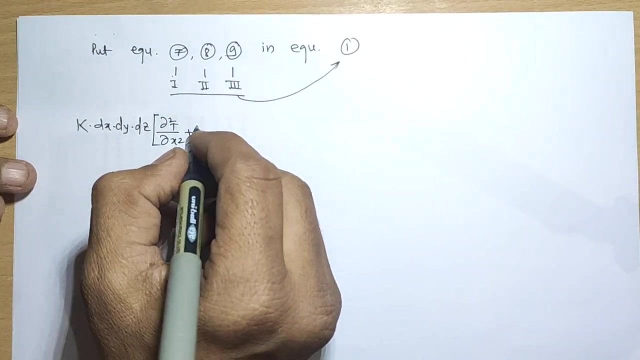 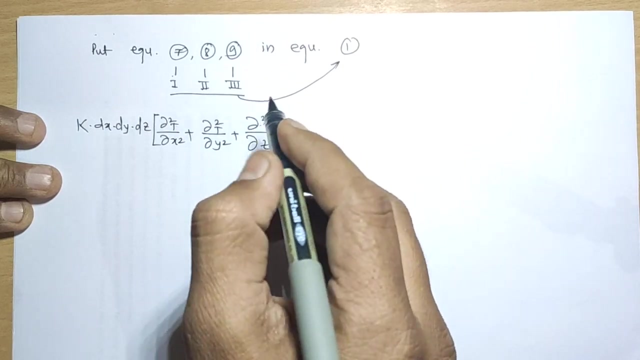 one that we have already derived, that k, k, d, x, d, y, d, z that you can refer just now, we have proved daba square t, daba x square plus plus daba square t, daba y square plus daba square t, daba z square. that's the equation number seven and part number one plus daba. 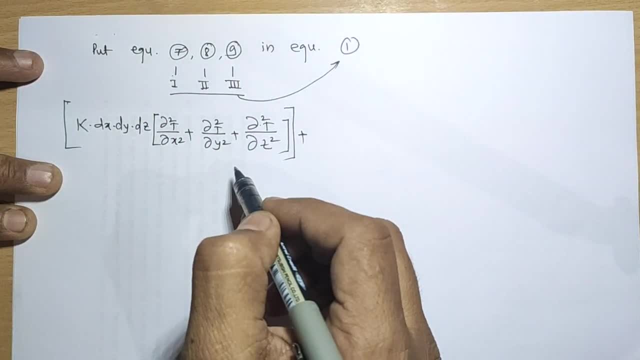 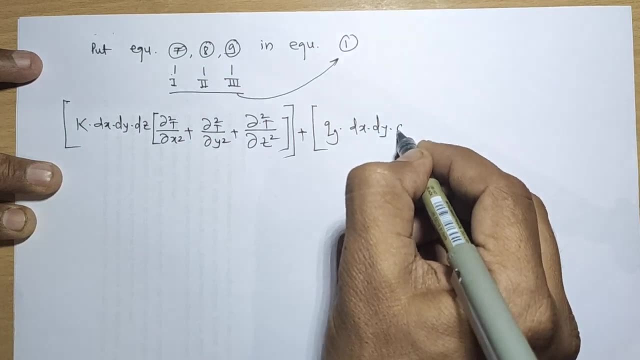 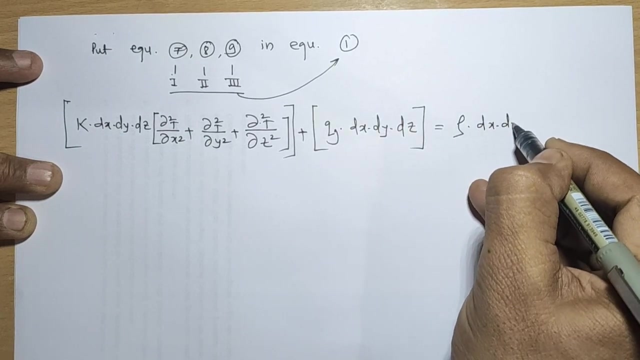 square plus. so this is part number one. what is part number two? part number two is heat generated and which is nothing but q, g, d x, d, y and d z. that is, the part number two is equal to part number three. what says part number three? part number three is d x already. 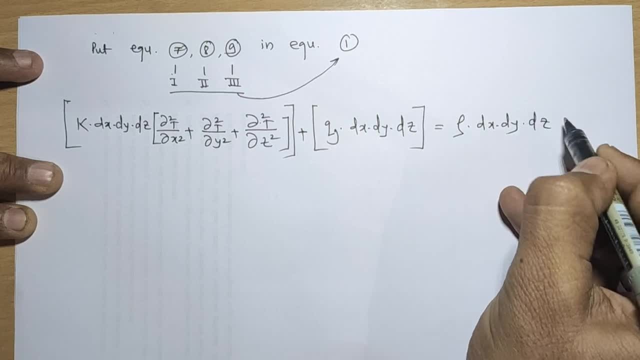 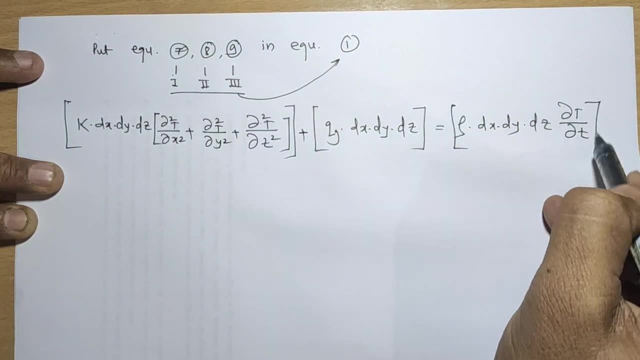 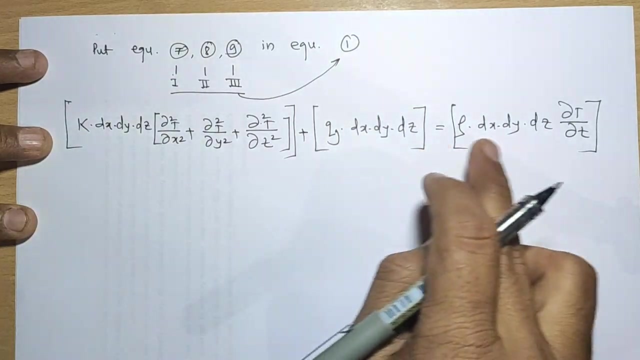 we have derived equation part number one, two, three, d, x, d, y, d, z, daba t, y, daba t. so these three parts, we have got it and we have put into equation number. now we have to simplify this. we have to simplify this from all three bracket: bracket number one, two and three. what? 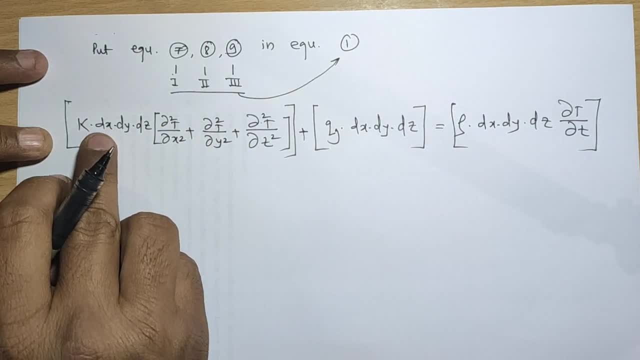 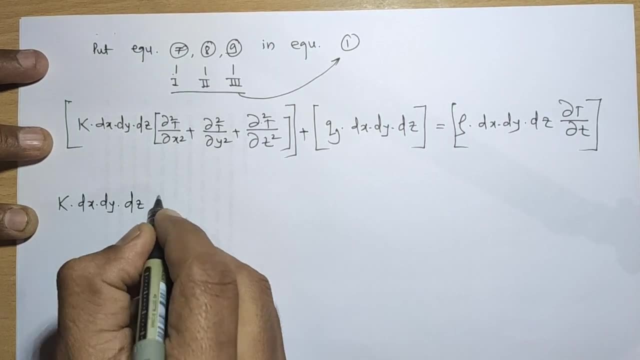 i am going to take. i am going to take common as a k d x, d, y d z. so if i take common as k d x, d y d z, what will be inside the bracket from this? if i take k d x, d, y d z, so what? 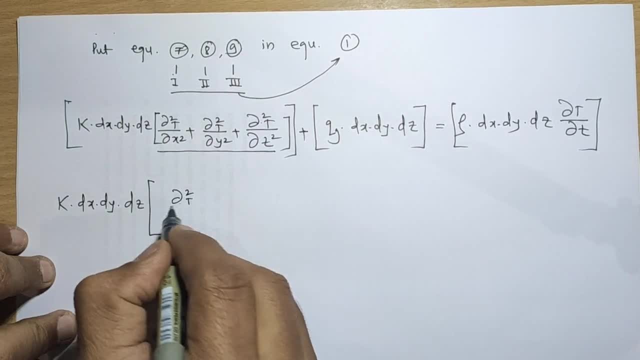 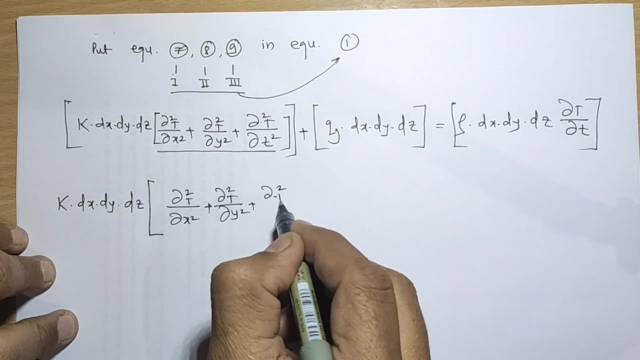 is remaining. remaining is this term, so i will write as a: daba square t daba x square plus daba square t daba y square square plus daba square t daba z square. this is what first term we have got plus from this. 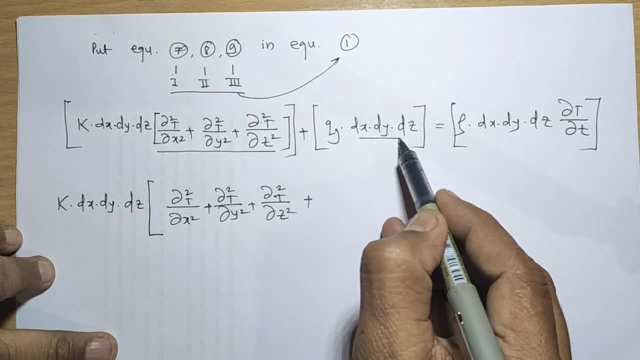 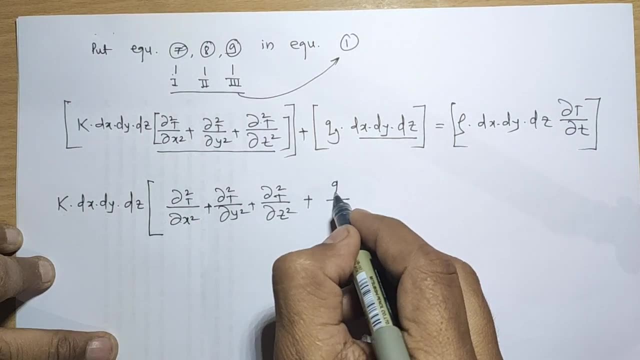 if i take common as a k dx, dy, dz, dx, dy dz is already present there, but k is not present there. so as k, we have taken common outside. so on, denominator k will be added and numerator qg is added from this, what we have taken common outside is k dx dy dz. okay, so this is from. 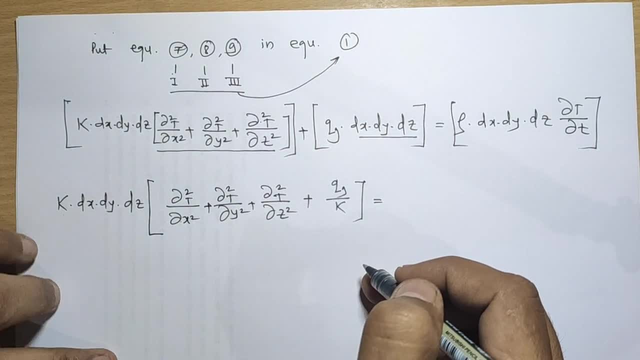 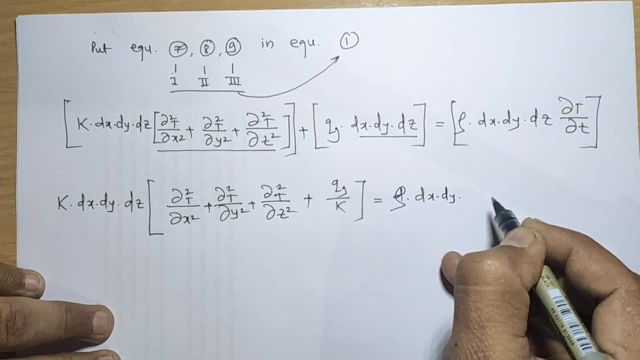 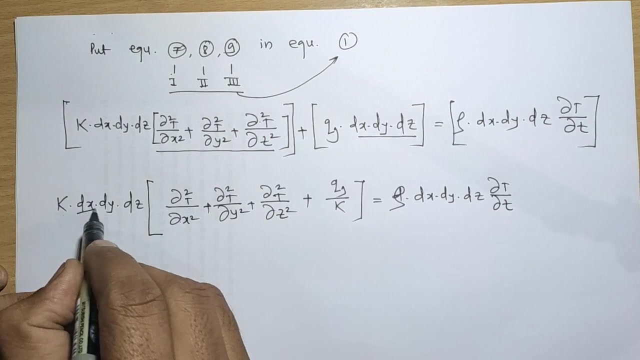 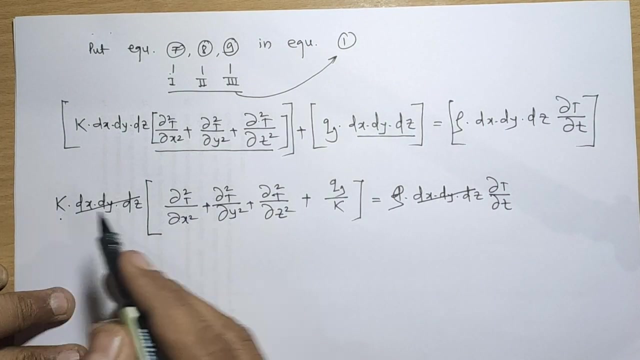 right side, from left side, from left side. i will take, i will write as it is: rho dx dy dz, dot by dot. this is what equation now this dx dy dz and dx dy dz can be cancel and this k, this k, cp is remaining here. rho cp, this is cp. 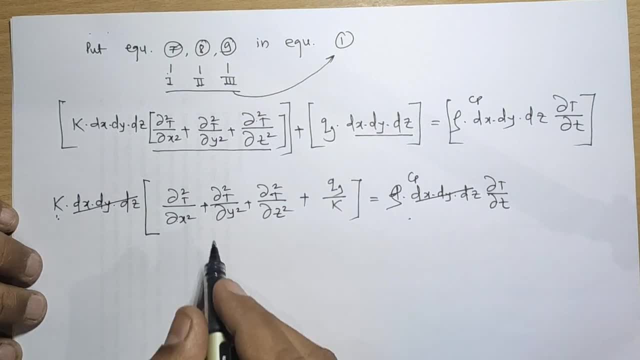 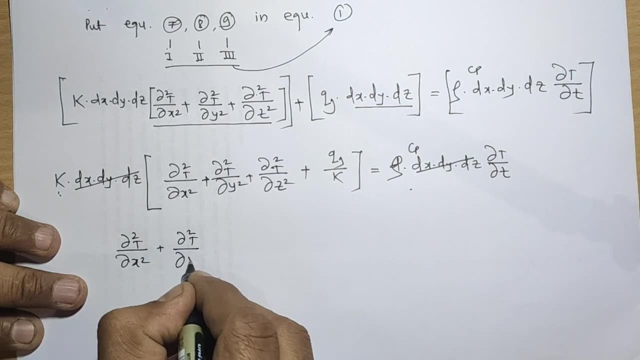 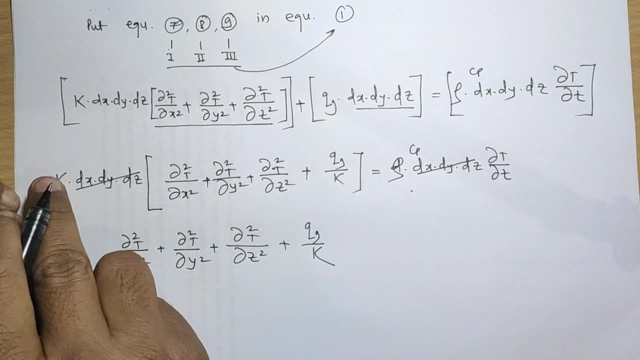 okay, so. So this k I am going to take on this side. So what will be equation now? The equation will become: daba square t, daba x square plus daba square t, daba y square plus daba square t, daba z square plus qg by k, This k I am going to take on this side. So it will become: 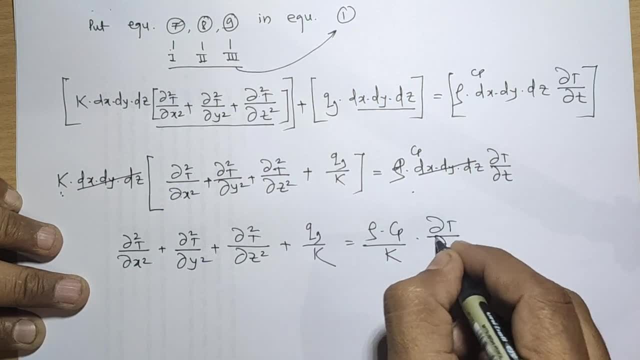 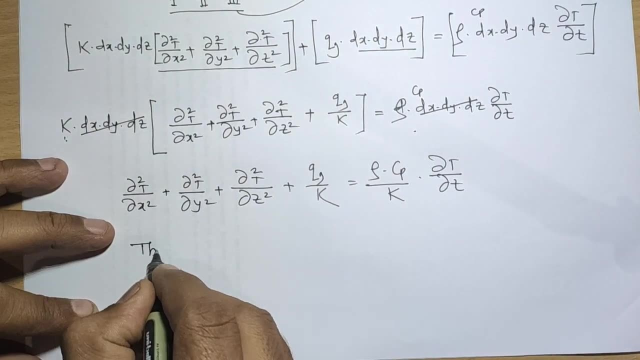 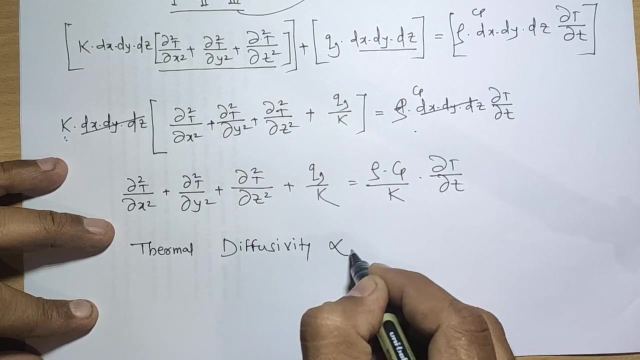 rho cp by k into dou t by dou t. That's the equation we have got here. Now I am going to introduce new term, that's what called as thermal diffusivity In the heat transfer. there is one term, that's what called as thermal diffusivity, which is denoted by alpha and.